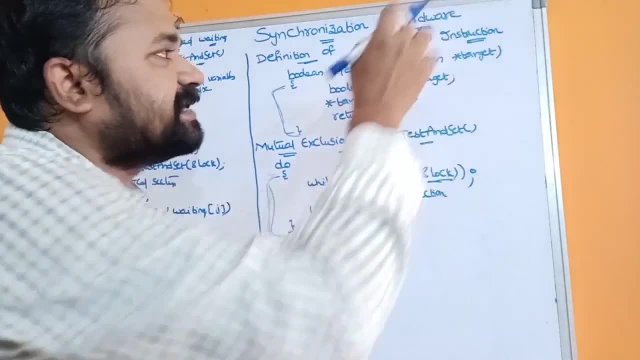 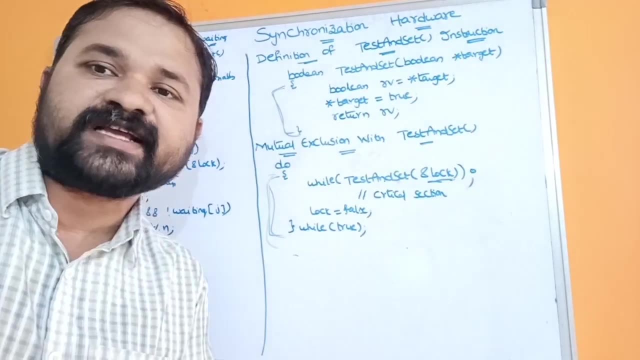 also Here it is a mission instruction. Test and set is nothing but a mission instruction. We know what is a mission instruction. It is in the form of zeros and ones, But for our understanding purpose we have written the code in the form of C language. Here, test and set is nothing but. 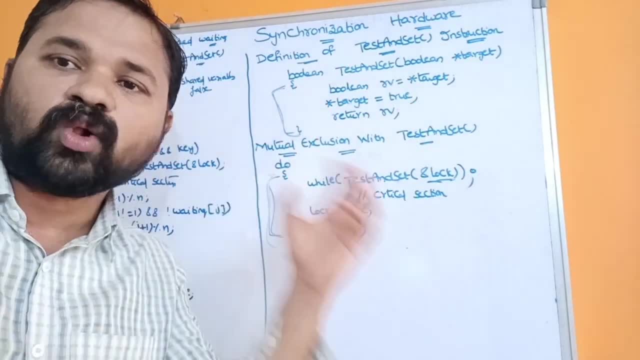 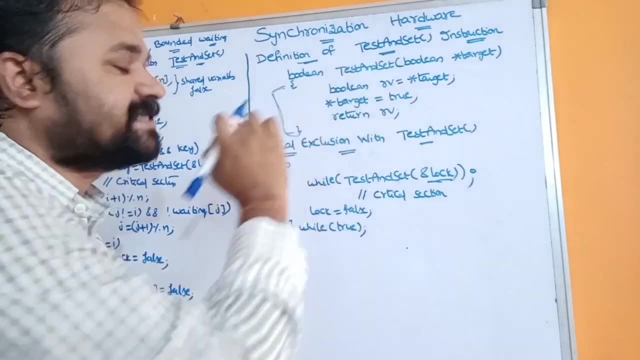 atomic instruction. We know what is atomic instruction. All the instructions are executed, yet once In the form of C language. we have written the code in the form of C language. We have written in one mission cycle Here. test and set contains one, two, six instructions. So all these six. 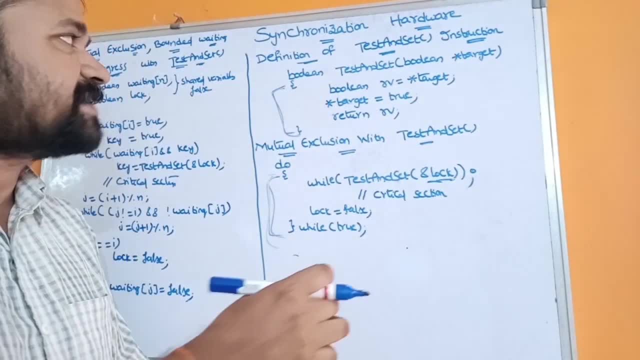 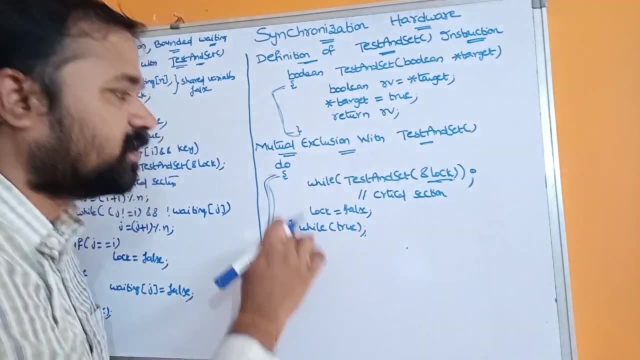 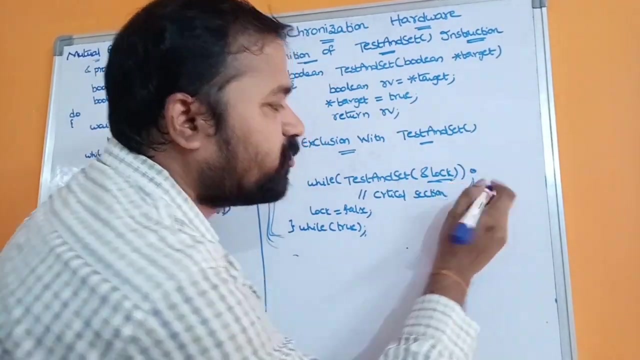 instructions will be executed in one mission cycle. Now let us see how we can achieve mutual exclusion with the test and set instruction. Here we are using some do by loop. So while test and set of yamper cent log semicolon, Here we are using semicolon. If we use a semicolon. 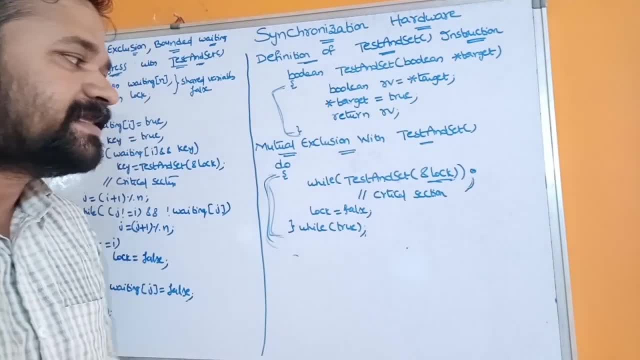 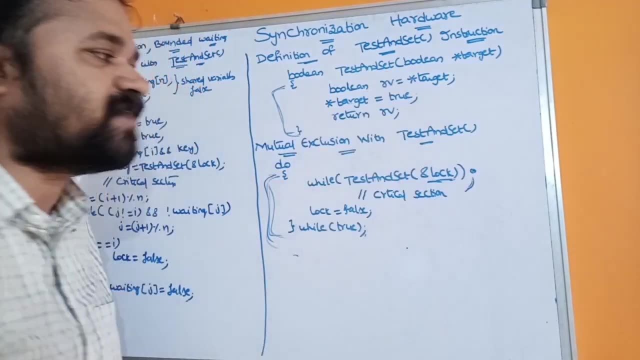 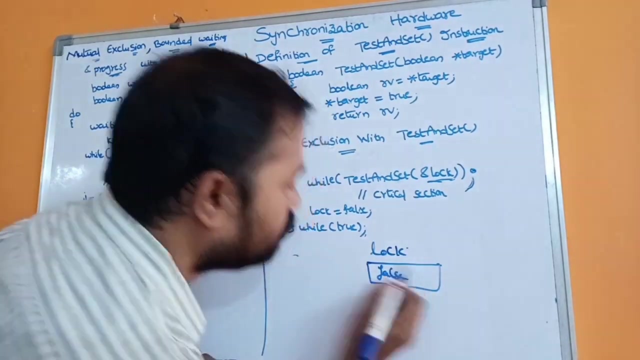 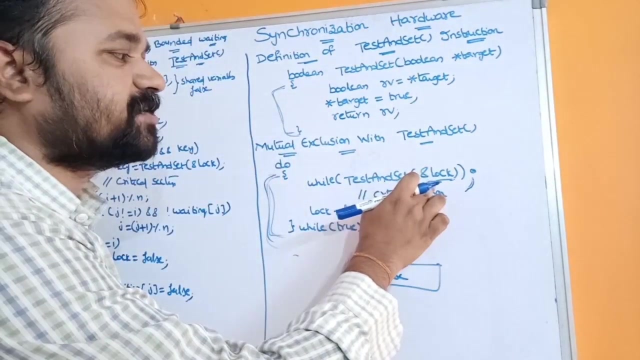 at the end of the by loop, then if the condition is true, then the while. then the control will stay in the loop. Here the initial value of the log is false. So while test and set of yamper cent log, let address of the log is 1000.. So whenever the statement is executed, then the control goes. 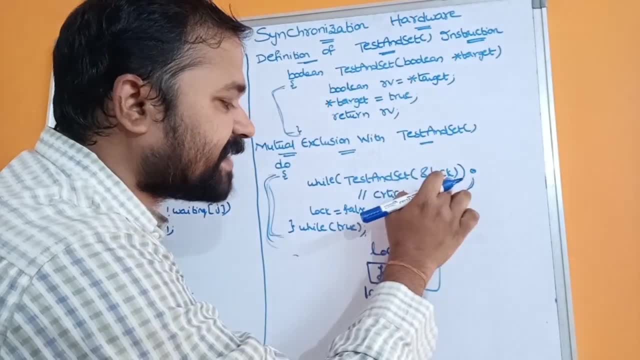 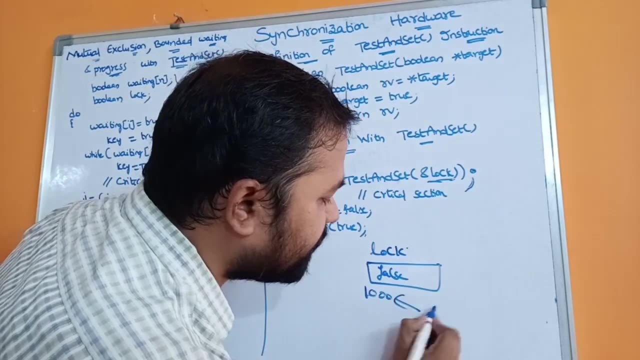 to the test and set function. So what is the address here? Yamper cent log means 1000. So this 1000 will be passed to the target. So now that means log and target are the same. Target are pointing to the same memory location, that is 1000.. So if you perform any modification, 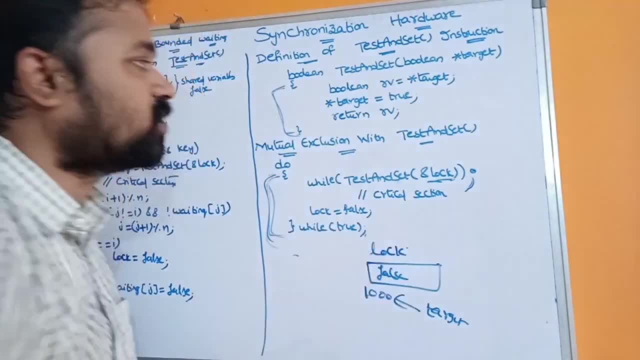 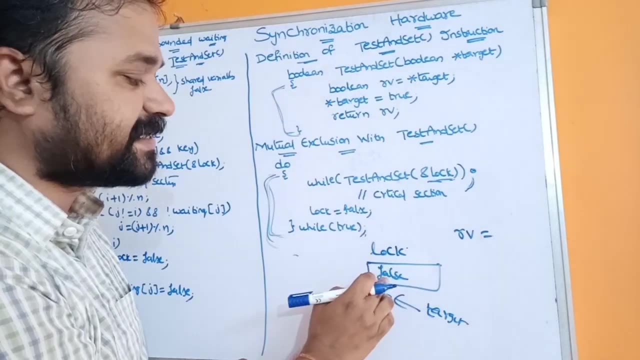 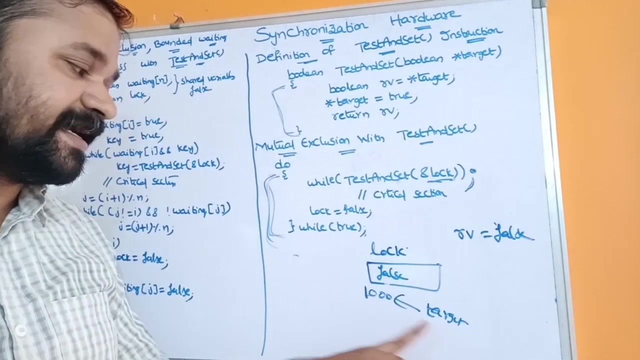 on target, then that modification will be reflected on log. also, Boolean rb is equal to star target, So rb is equal to. So what is the value it is getting False? So rb is equal to false. Next, star target is equal to true. So this is target. Target means 1000.. So star 1000. 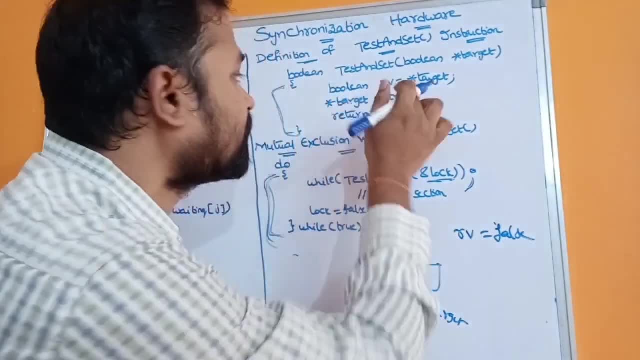 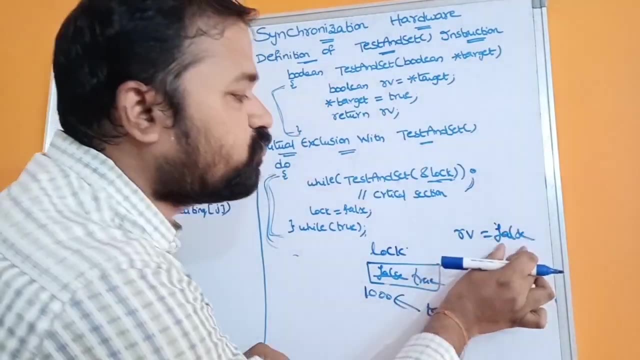 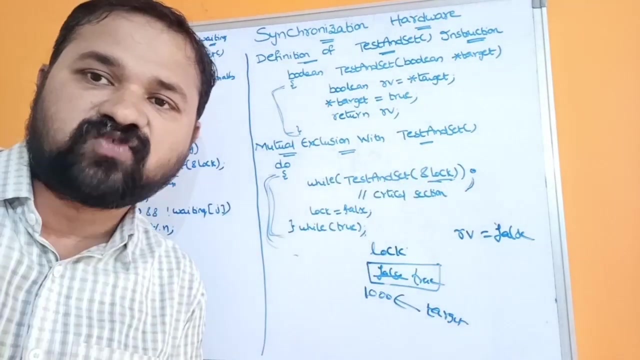 means value at log. So now the value will become what True? True, Next written rb. So what is rb False? So now false will be written, and here the false will be substituted. Here the result is false. So by now false means false. So here: 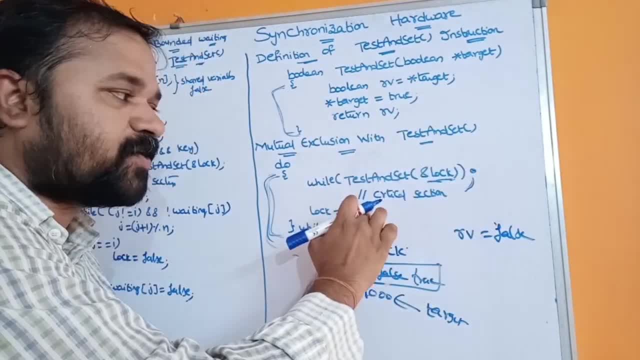 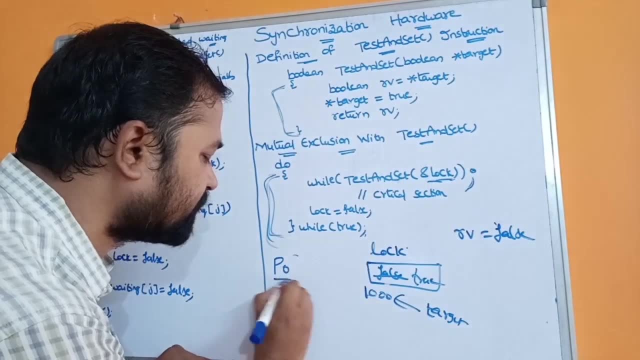 the condition is false. So whenever the condition is false, then the control comes out from the value. So now p0 is in Let. the first process is p0.. So now p0 is in critical section. So whenever p0 has completed all its operations, 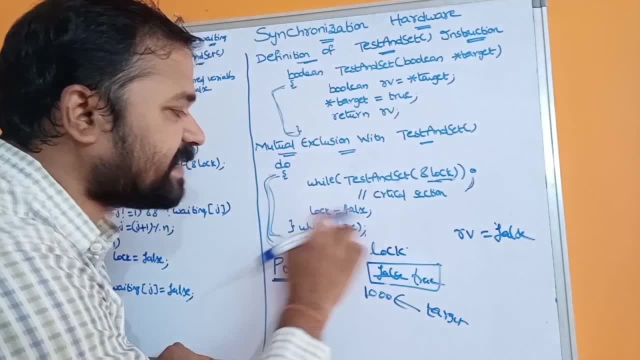 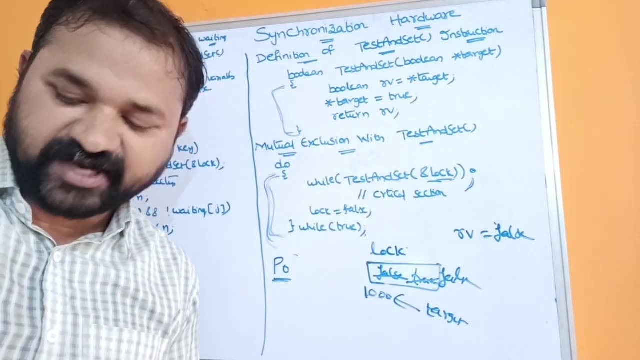 Then p0 comes out from the critical section and it places here as log is equal to false. So if log is false, then other process can enter into the critical section, Such as p1, p2, p3. all those processes can enter into the critical section. Now let us check whether 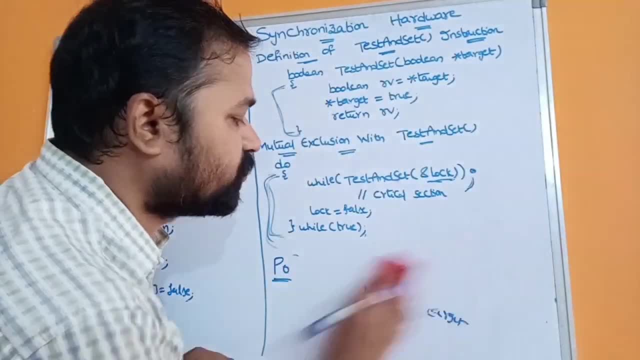 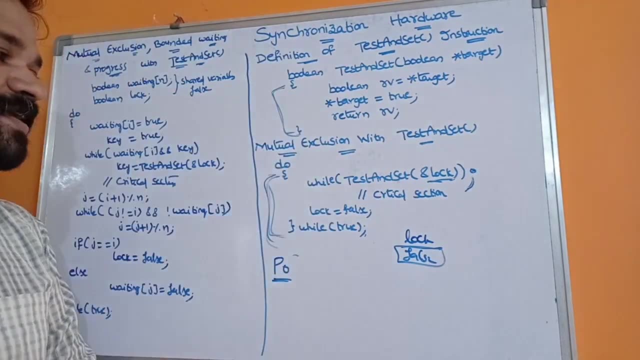 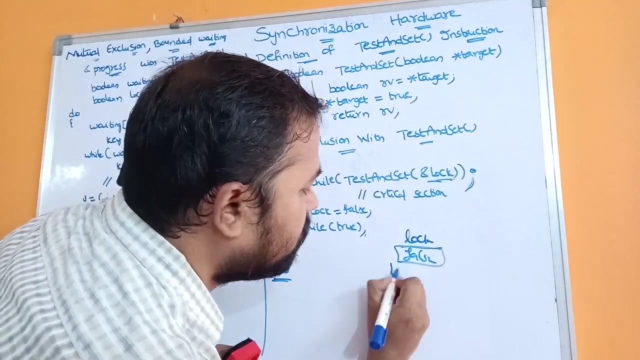 it is satisfying mutual exclusion or not. So initially, what is the initial value of the log? The initial value of the log is false. Let p0 wants to enter into the critical section, So we will use this value. So while test and set of ampersand log. So what is log Ampersand? 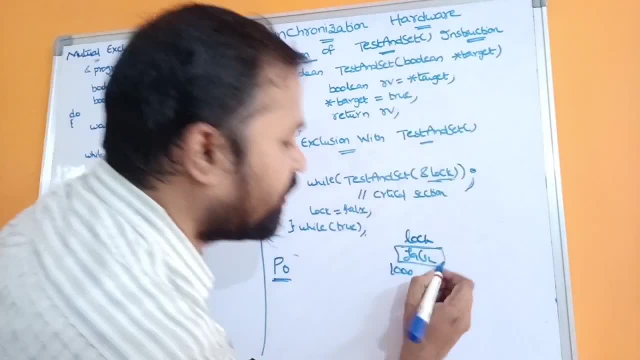 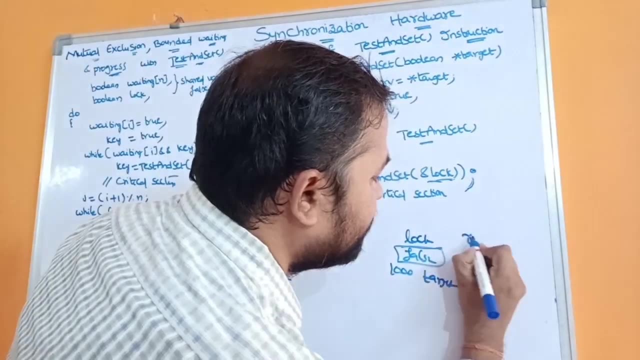 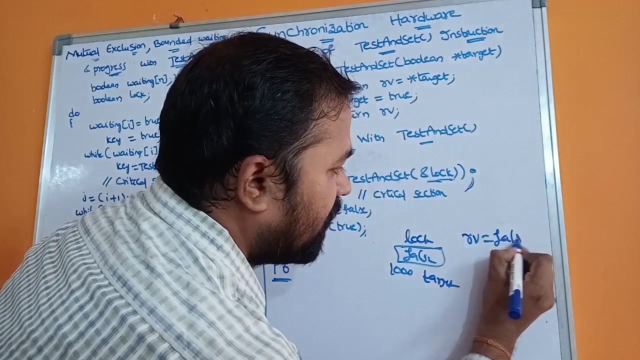 log means ampersand 1000.. So this 1000 will be passed to the target. Now log and target: target 1000: memory location. Next boolean: rb is equal to star target. So what is rb? Target means 1000. Star 1000 means value at 1000. That is false. rb is equal to false. 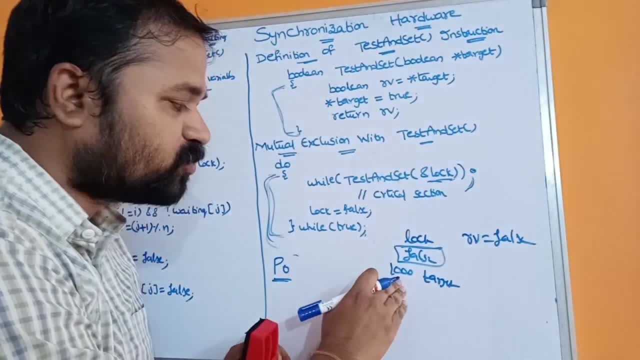 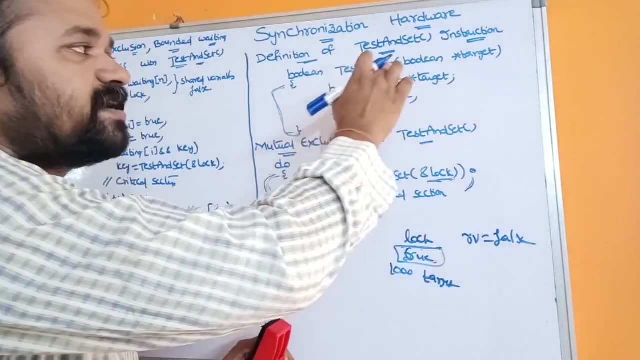 Next, star target is equal to true, So target means 1000.. Star 1000 means The value at the 1000.. So now what we are doing? We are making this as true. So that is why it is called yes, test and set, So test the instruction and set. So set means making. 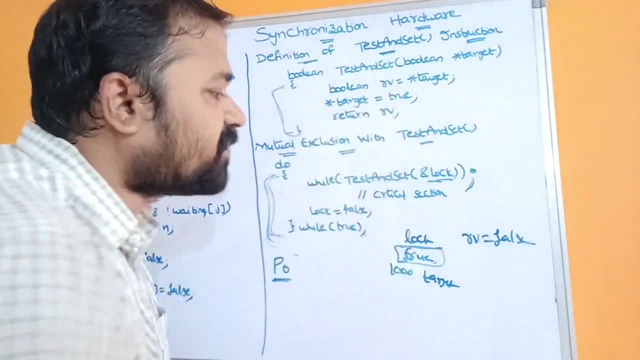 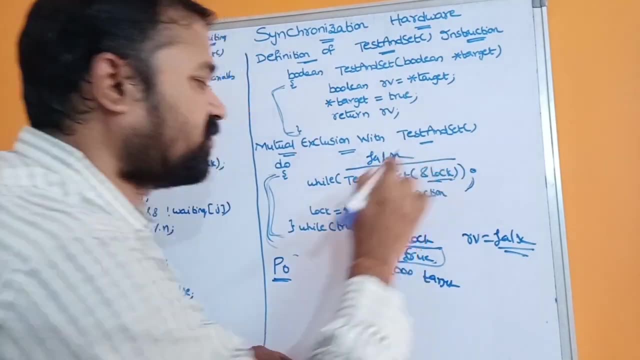 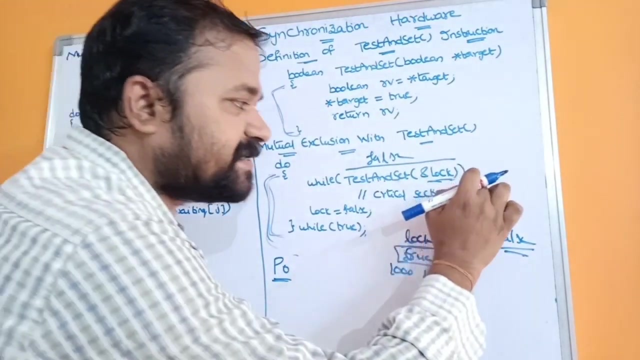 that value as true. 1 set means 1. Return rb. So what is rb value? False, So now false will be returned. Now, this result is false. This result is false. So while of false, semicolon. So while of false means what False? So condition is false, But here we place a semicolon, So 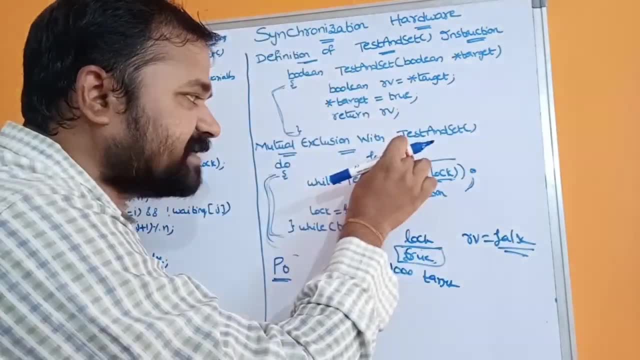 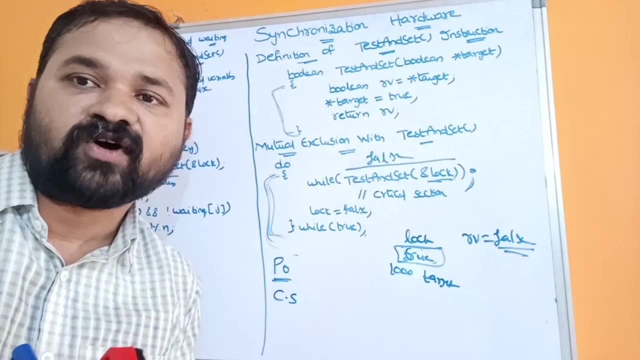 whenever we place a semicolon- So here we place a semicolon, So here we place a semicolon At the end of the while loop- Then whenever the condition is false, then the control comes out from the while loop. Now p0 is in the critical section. Let us assume that. now p1. 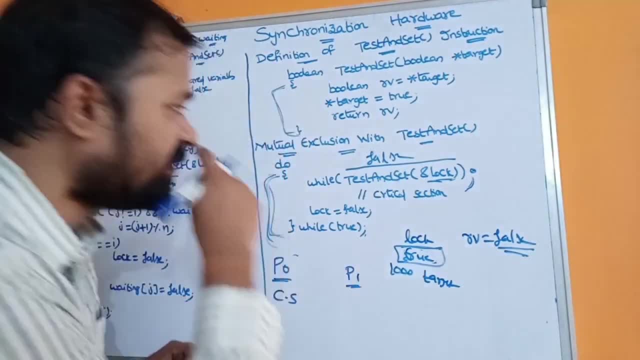 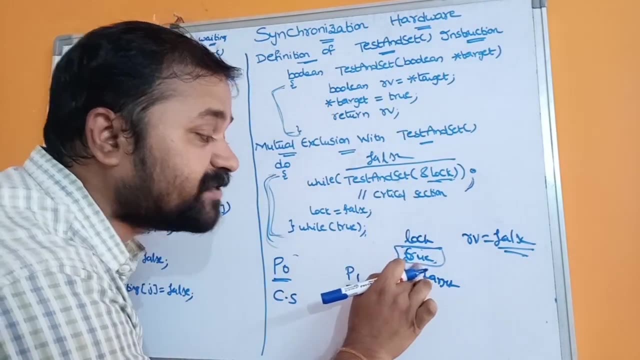 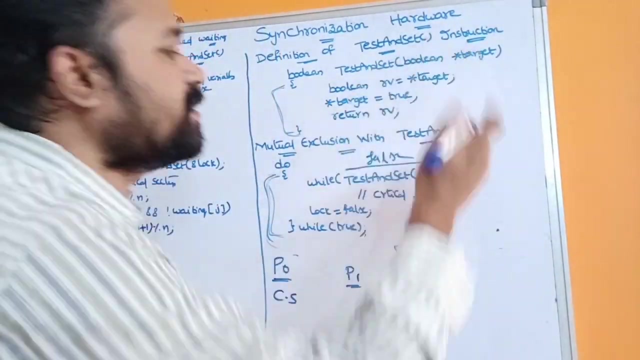 wants to enter into the critical section. So for that first p1 has to execute this while loop, While test and set of yamper sent log. But what is log now? Log value is true. So now control goes to the test and set. Now what is target? True Boolean rb is equal. 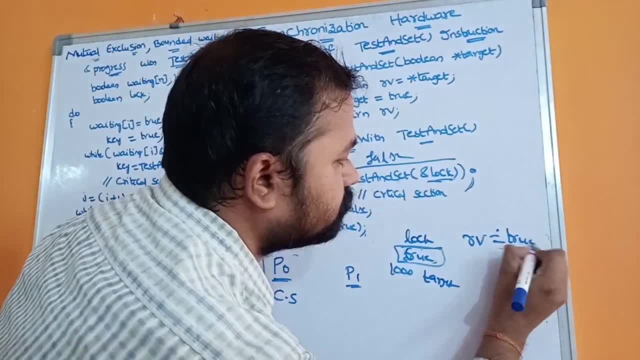 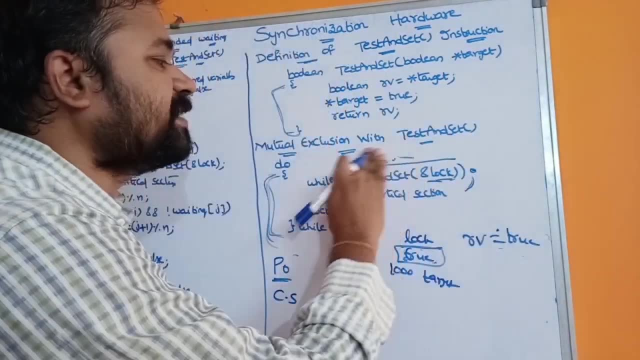 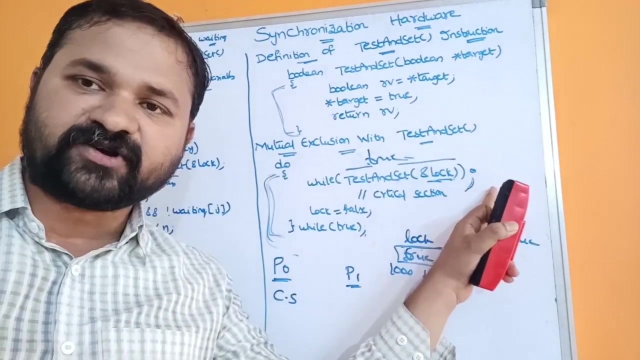 to star target. So what is the value? Target: true. Next star target is equal to true. Already it is true. only Return rb. So now what will happen? True will be returned and it will be substituted here, So while of true. So while of true means condition is true. But here we place a semicolon. If 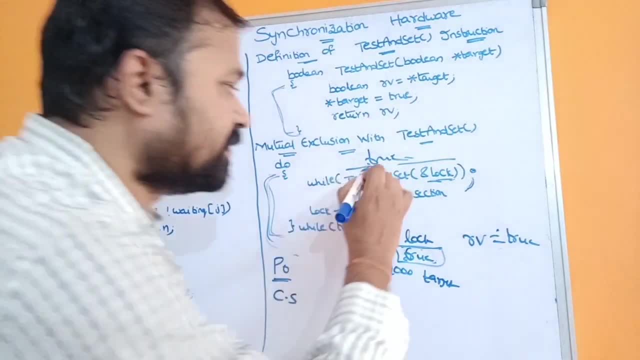 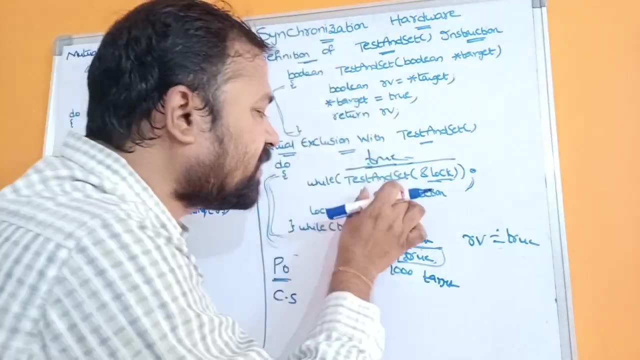 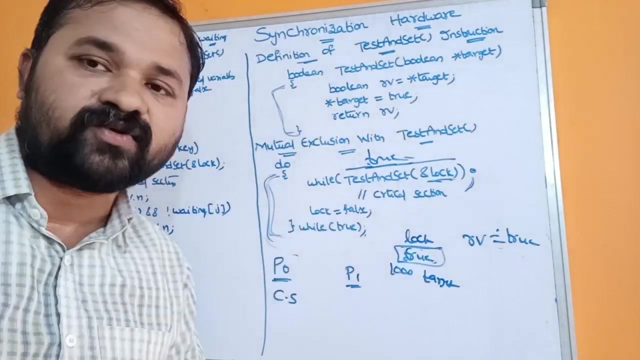 we place a semicolon at the end of the while loop, then what will happen Then? whenever the condition is true, then the control remains in this while loop only. So now, p1 will stay in this while loop only Whenever the log will become false. So as long as log is true, value p1 will stay in. 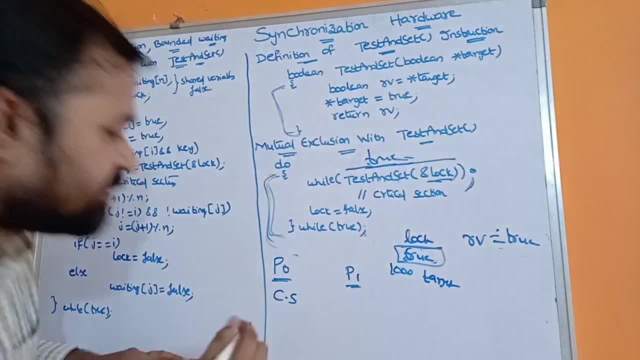 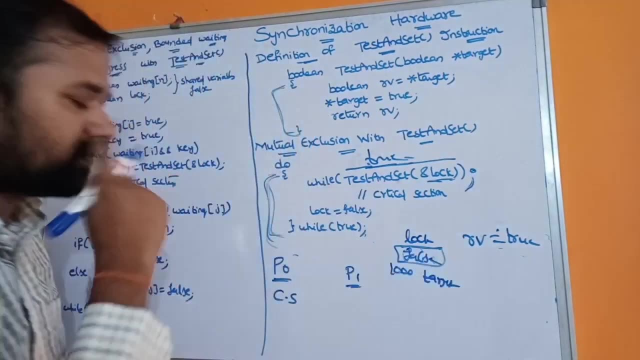 this while loop only. So whenever p0 comes out from the critical section it makes log as false. Let p0 comes out from the critical section. Now p0 can make log as false. Now p1 can enter into the critical section. So here it is satisfying mutual exclusion We. 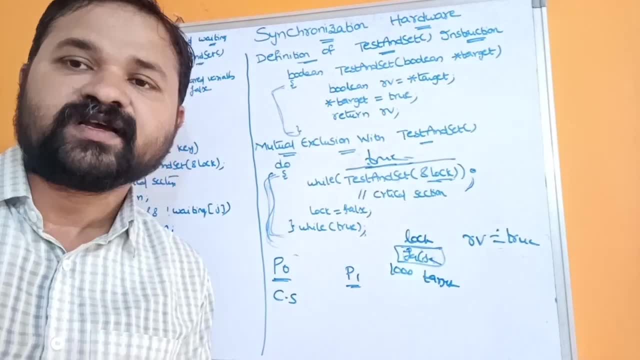 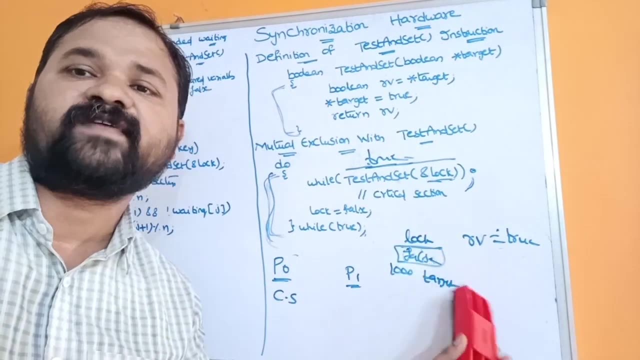 know what is mutual exclusion. When one process is in the critical section, then no other process is allowed to enter into the critical section. when P0 is in the critical section, then we are not allowing P1 to enter into the critical section. So we can say that this is satisfying mutual exclusion. Now let us check whether 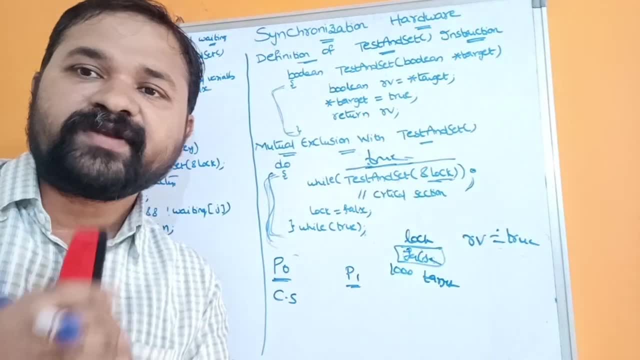 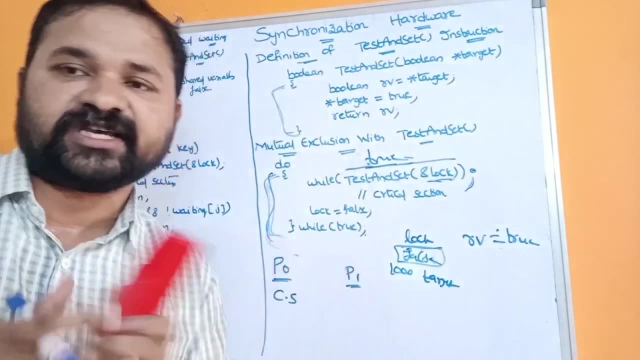 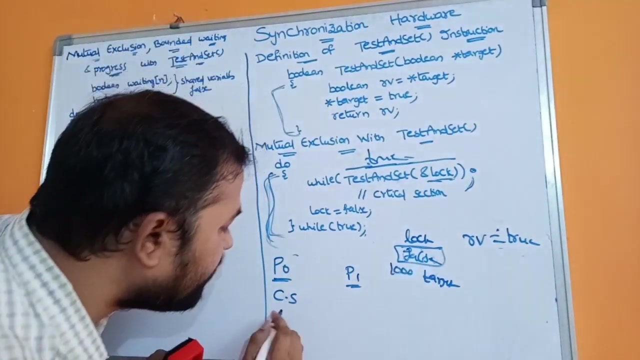 it is satisfying bounded weighting or not. So bounded weighting means each process must get a limited number of chances in order to enter into the critical section. This should not give more chances for a particular process. Let us assume that now P0 is in the critical. 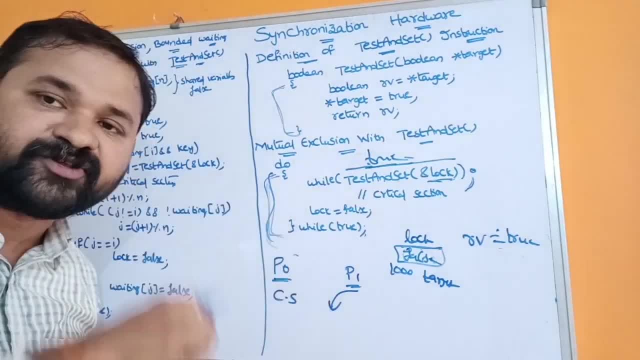 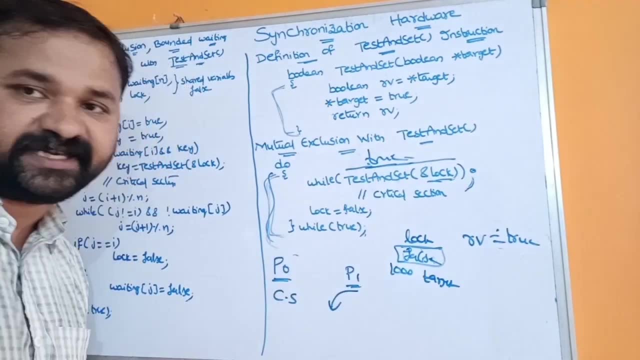 section and P1 is waiting for entering into the critical section. So here, what is the point? P0 is in the critical section and P1 is waiting for entering into the critical section. After comes out from the critical section, let us assume that P0 has put one. 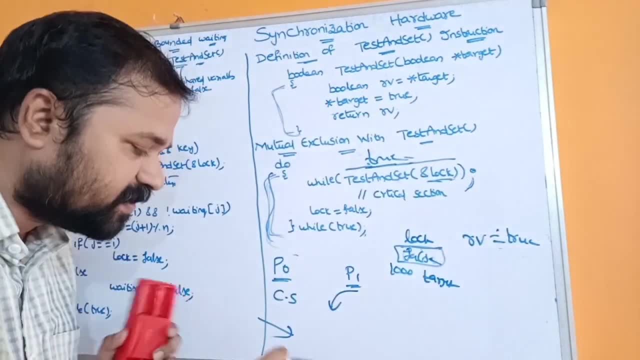 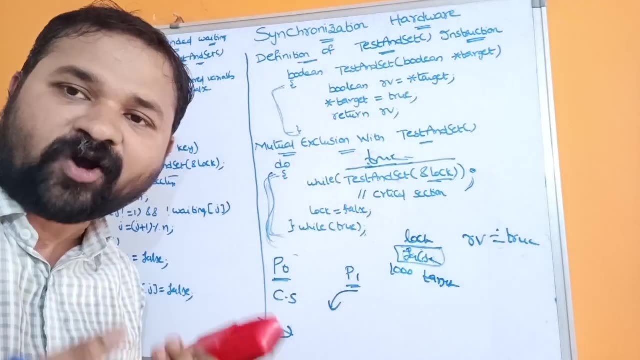 more request to enter into the critical section. So now, what is the point? P0 is trying to enter into the critical section as well, as P1 is trying to enter into the critical section, but assumes that operating system has given chance for P0.. 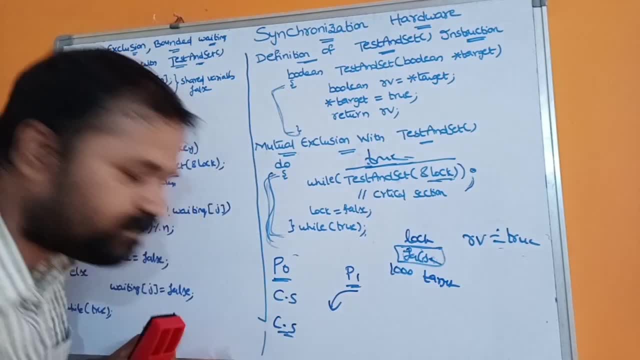 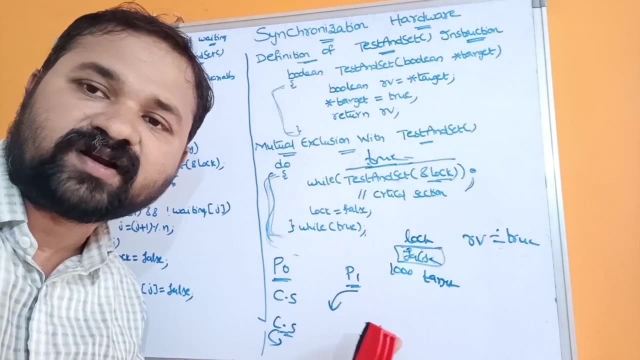 Okay, so now P0 will be in the critical section one more time After some time. also, P0 comes out from the critical section. assumes that P1 is waiting for entering into the critical section. Now, P0 and P1 both are waiting for entering into the critical section. 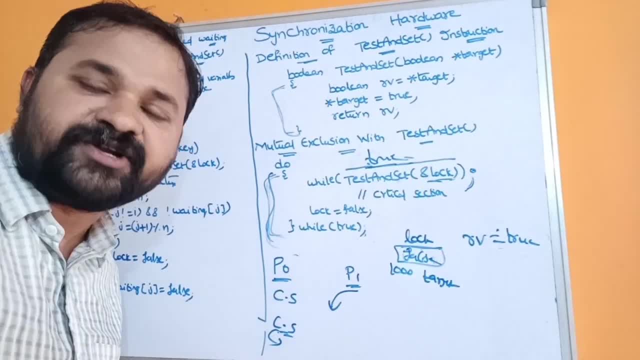 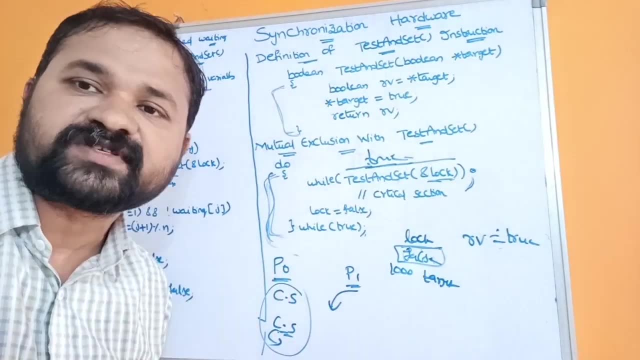 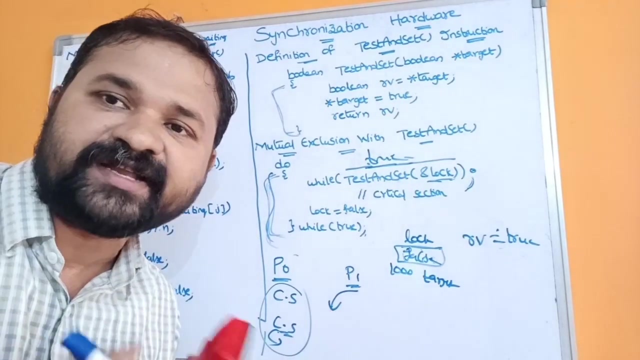 But assumes that operating system has given chance for P0 to enter into the critical section. So that means here what is happening? bounded waiting means there should be some limit on number of times a process can enter into the critical section. But every time here P0 is entering into the critical section, P1 is not getting any chance to enter into the critical section. 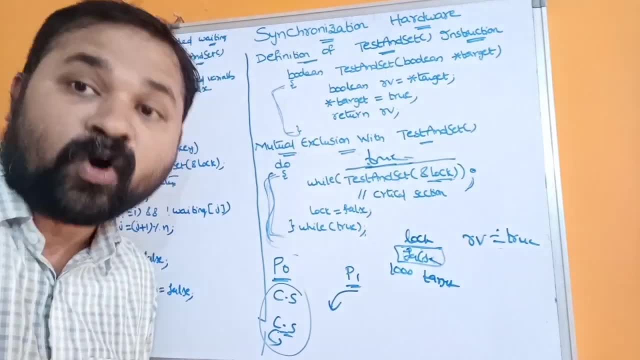 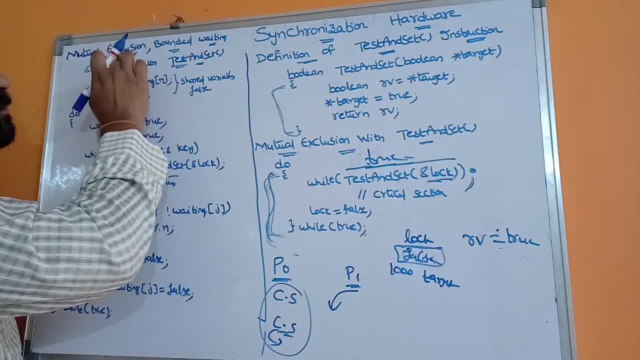 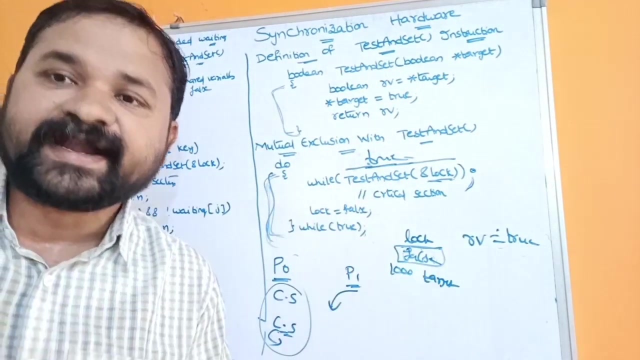 So we can say that this algorithm is not satisfying bounded waiting. So in order to overcome this problem, we are using one more algorithm. So this algorithm will satisfy mutual exclusion, bounded waiting and progress. So we know about critical section. Any solution to the critical section must satisfy three requirements. 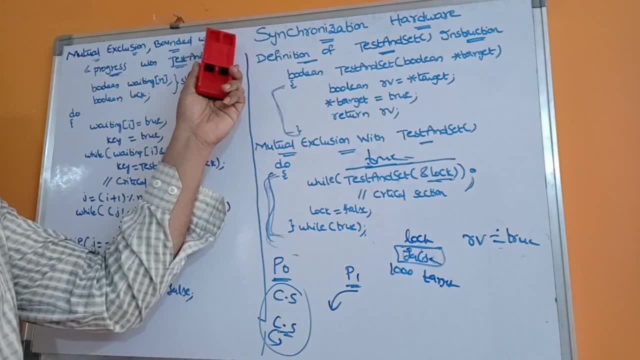 The first requirement is: First requirement is mutual exclusion. Second requirement is bounded waiting. Third requirement is progress. It is satisfying only mutual exclusion. It is not satisfying bounded waiting as well, as it does not satisfy progress also. But we should not bother about progress. 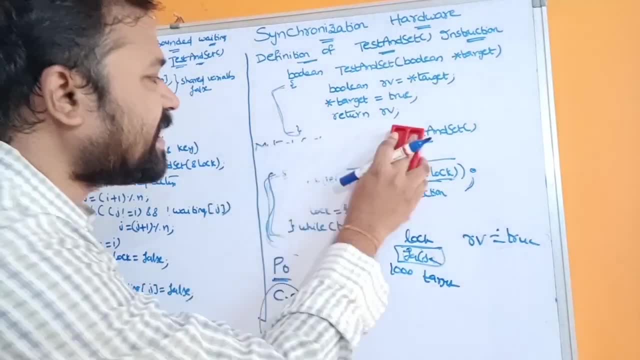 Why? because it is not satisfying bounded waiting. If it is not satisfying bounded waiting, then it does not satisfy progress also. This algorithm will satisfy mutual exclusion bounded waiting as well as progress. also Here in this algorithm we have two requirements. First requirement is: 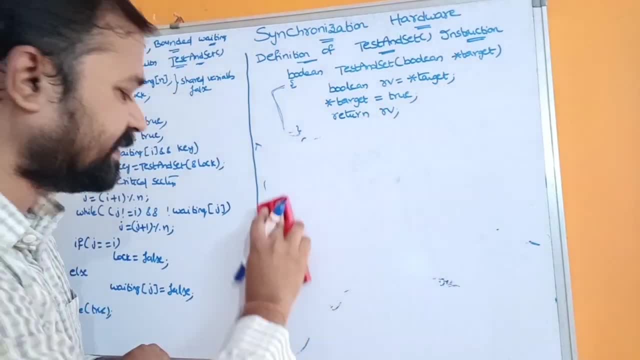 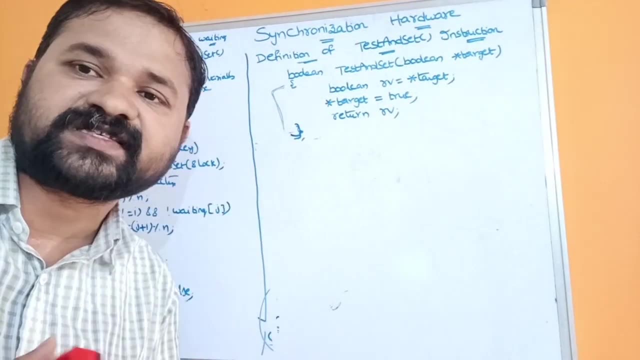 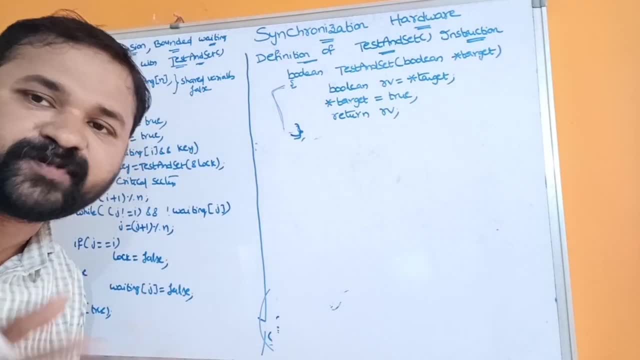 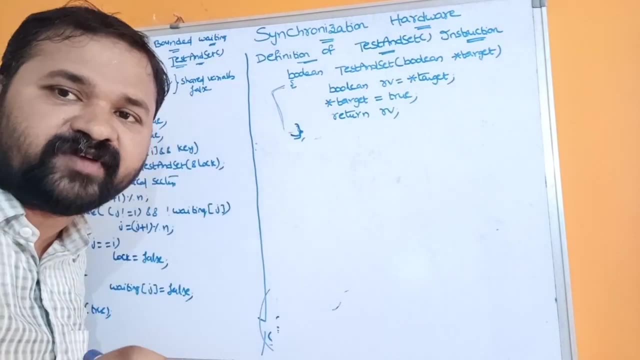 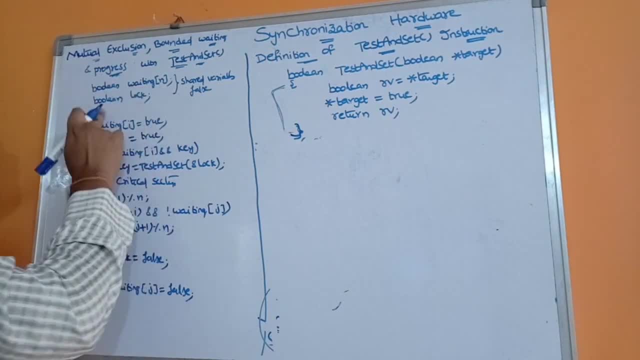 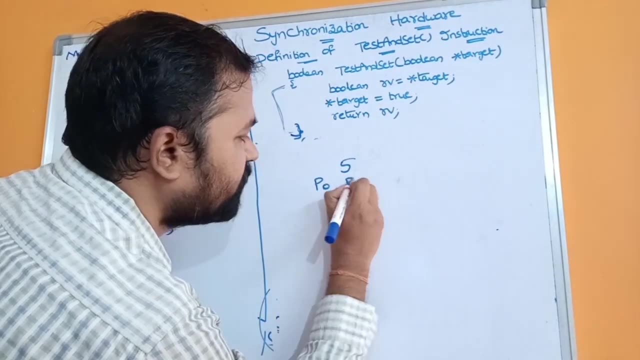 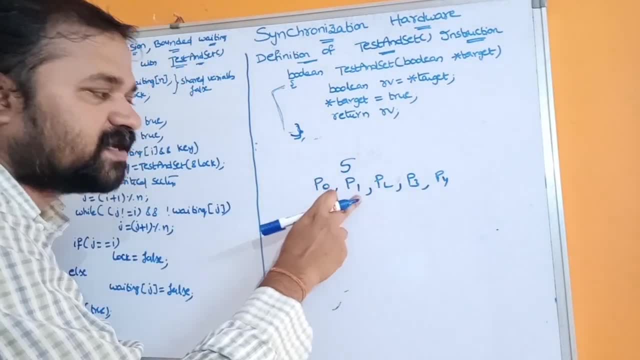 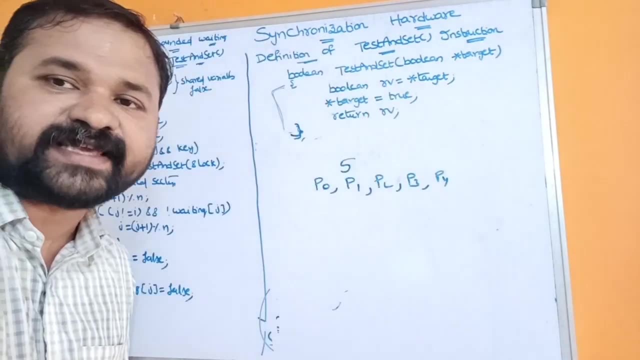 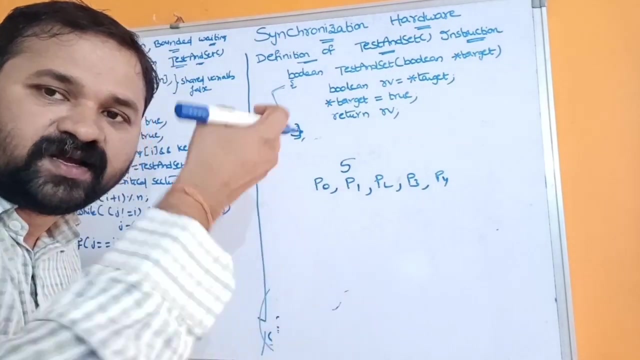 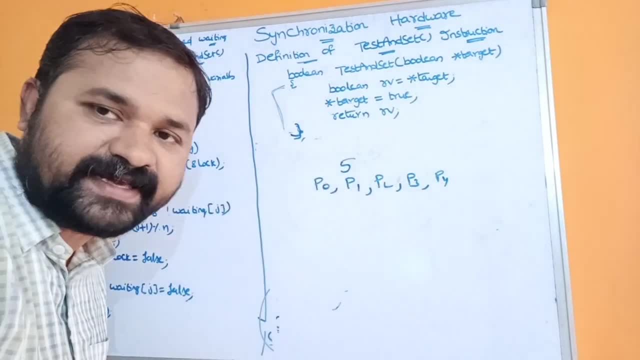 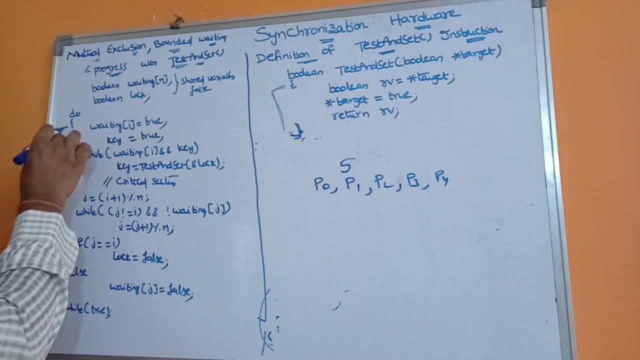 Suppose, if waiting of 2 is true, it specifies that P0 is waiting to enter into the critical section. Likewise, the initial value of the lock is also false. And now this is nothing but the code. here, In this algorithm also, we are using test and set instruction. 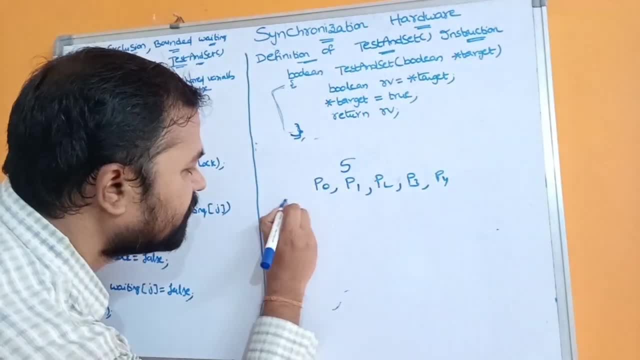 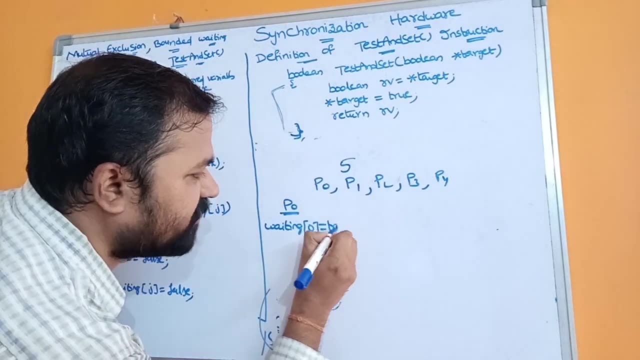 So waiting of i is equal to 2.. Let us assume that P0 wants to enter into the critical section, So it executes a statement for waiting of 0 is equal to 2.. So it specifies that P0 is waiting to enter into the critical section. 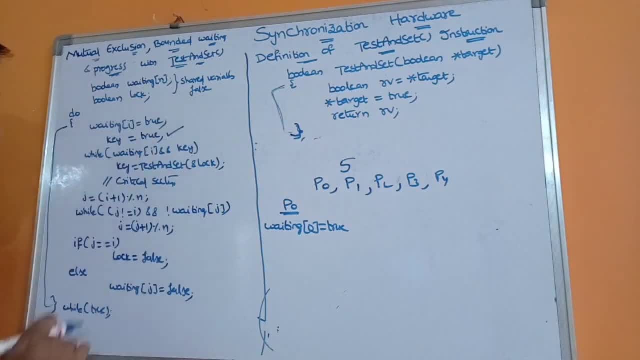 Next year. we are using two local variables. The first local variable is key, whereas the second local variable is j. So each process has its own local variable key. So key is nothing but the local variable, So key is equal to 2.. 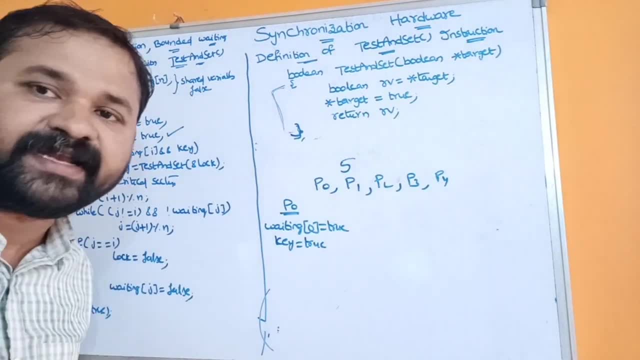 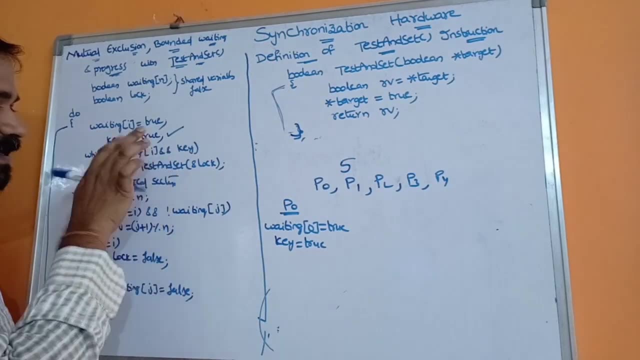 So it specifies that P0 process is waiting to enter into the critical section. Next, why waiting of i and key? Here we are using logical end. What is logical end? If both the conditions are true, then only the result is true. 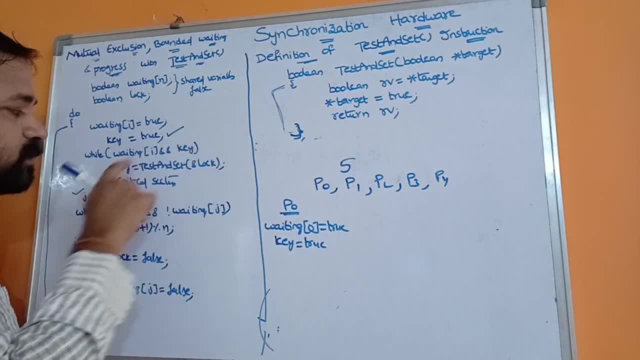 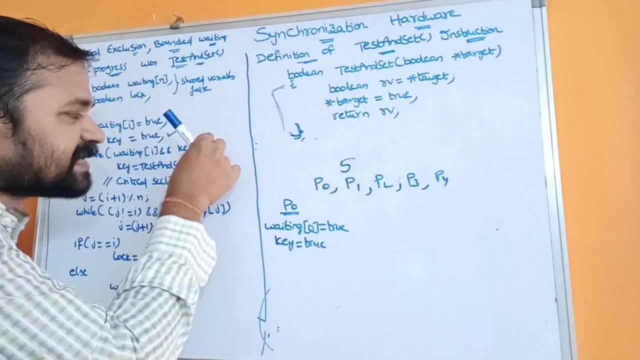 Otherwise the result is false. So when this condition is true, then we are going to execute this statement Here. there is no semicolon at the end of the while loop, So whenever this condition is false, then the control comes out from the while loop. 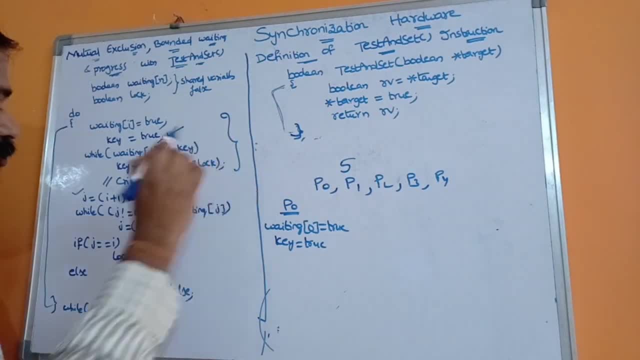 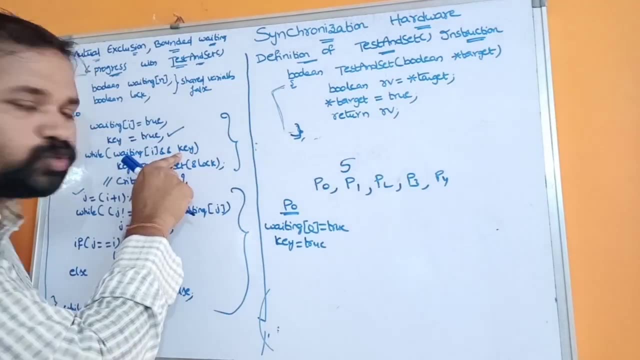 And we enter into the critical section. So this is nothing but entry section code, whereas all these statements are nothing but exit section code. So whenever this condition is true, then we can say that some other process is in the critical section. 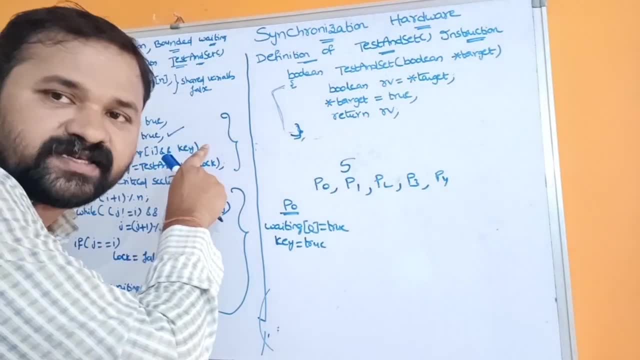 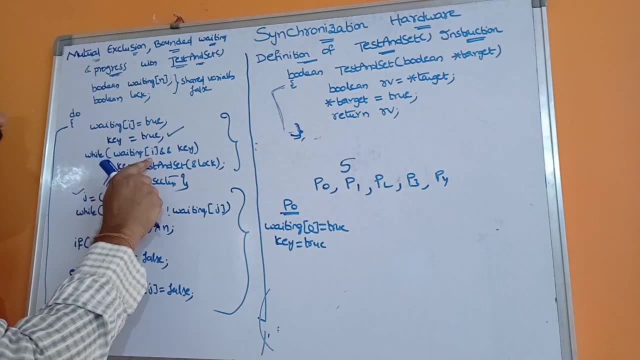 So that process has to wait. So whenever this condition is false, then only the control comes out from the while loop and that process will enter into the critical section. Now let us see this condition: While waiting of i. what is i now? 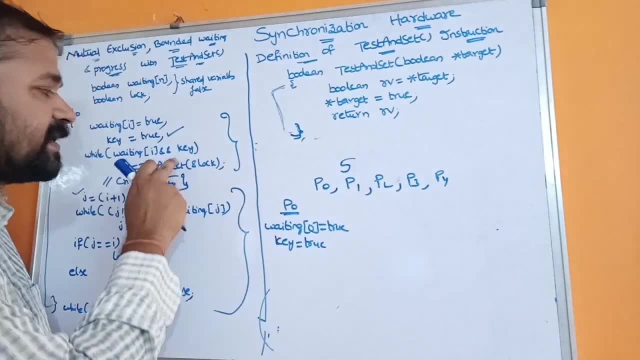 0.. While waiting of 0,, what is waiting of i, 0.. True Condition is true And key What is key, value True. So both the conditions are true. So that means the entire expression is true. 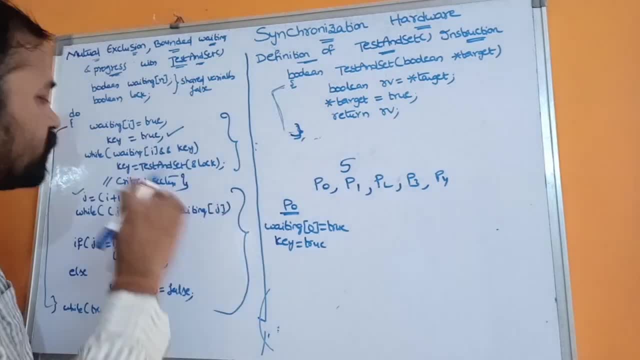 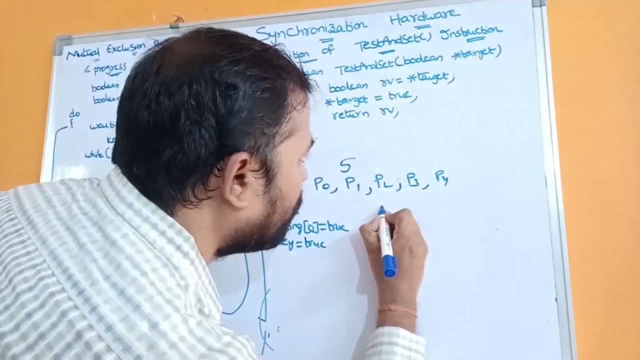 So while body wheel gets executed, key is equal to test and set of ampersand log Here. what is log value? What is log value? The initial value of the log is false. So here also we have to use a statement. 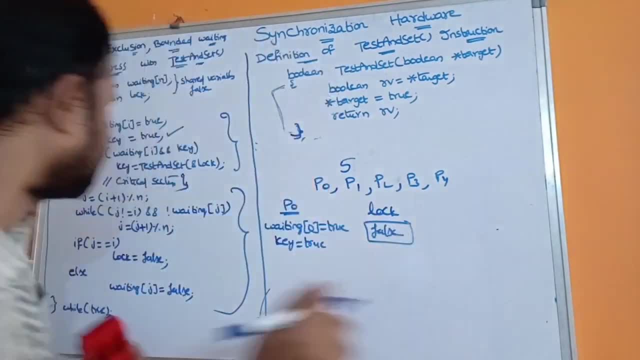 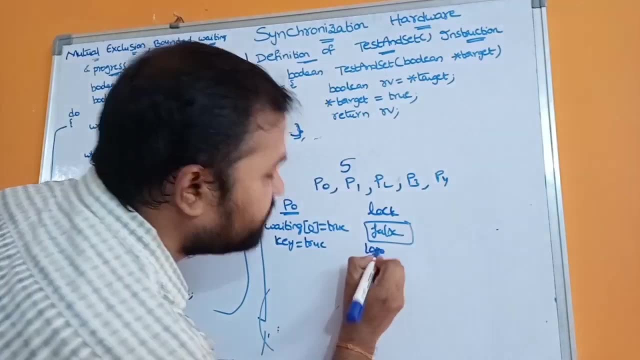 Name of the variable is log. The initial value of the log is false. So whenever this statement is executed, then the control goes to the test and set. So this address will be passed to target. Now log and target are pointing to 1000 memory location. 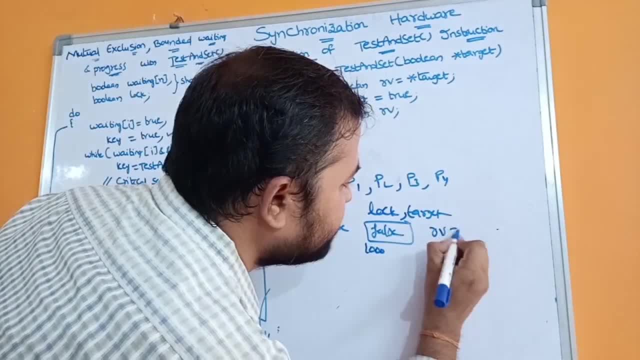 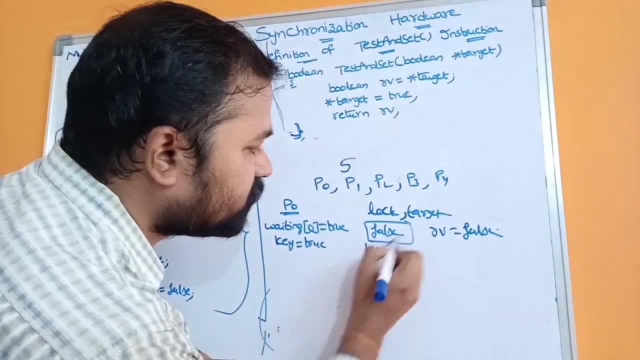 Next, rv is equal to star target, So rv is equal to what is the value in target False, So rv is equal to false. Next star target is equal to true, So target means 1000.. So 1000 means what? 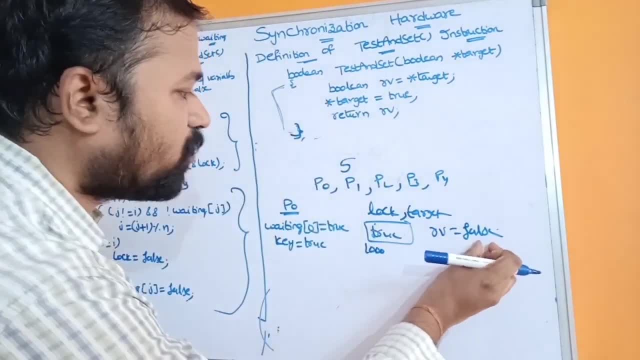 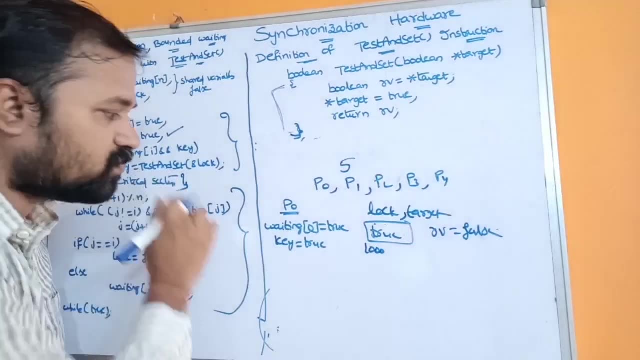 True, So place true here. Next written rv. So false will be written and it will be substituted here. It will be substituted here. Key is equal to false. Now, what is key? value False, So key is equal to false. 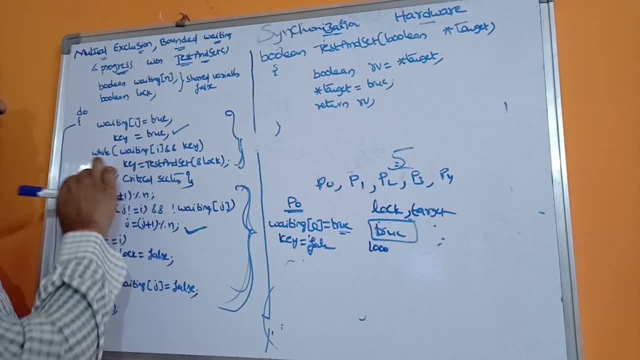 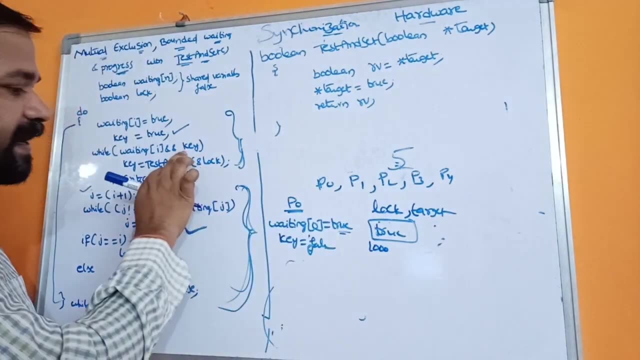 So this false value will be written here. So once again, control goes to the value, while weighting of 0 and key. So what is weighting of 0? True, And what is key value False. So true, false. 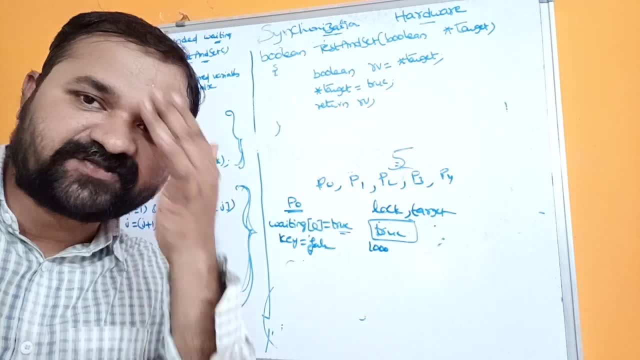 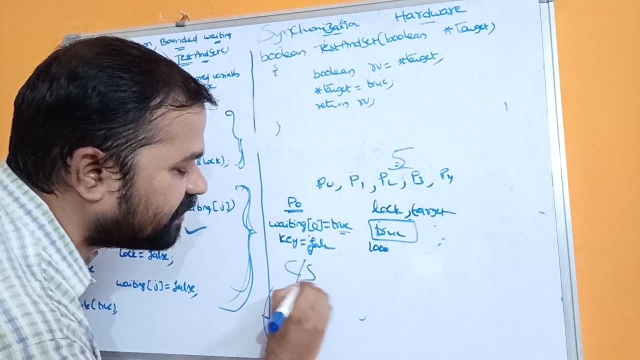 We know what is logical, and if one of the expression is false, then the entire expression will become false. So the control comes out from the value. So p0 process will enters into the critical section. Now let us check whether this algorithm is satisfying mutual exclusion or not. 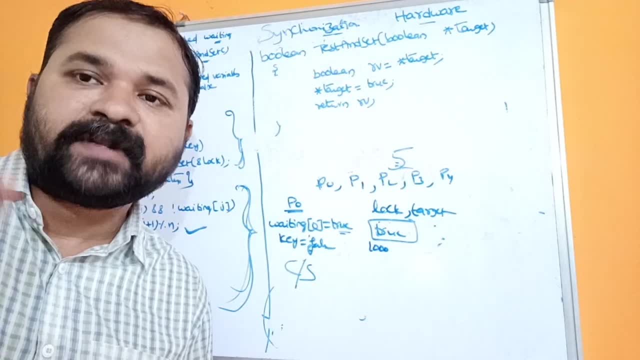 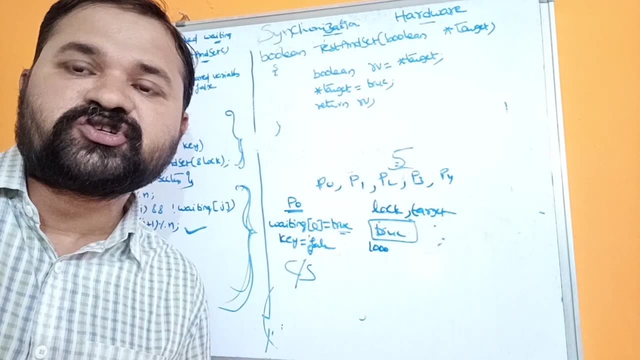 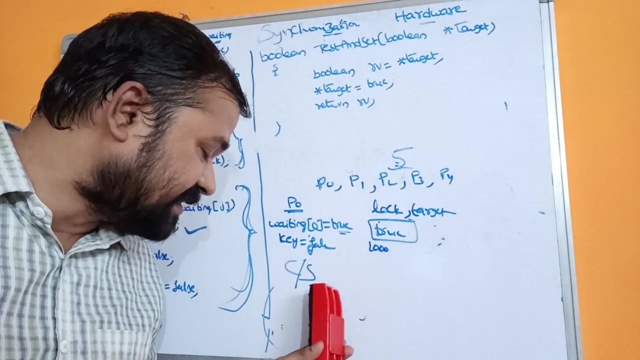 We know that any solution to the critical section problem must satisfy three requirements: Mutual exclusion, bounded weighting and progress. Let us see what is mutual exclusion. Only one process can enters into the critical section. When p0 process is in the critical section, then no other process is allowed. 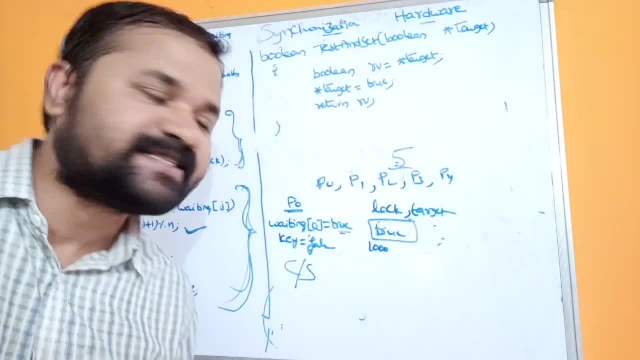 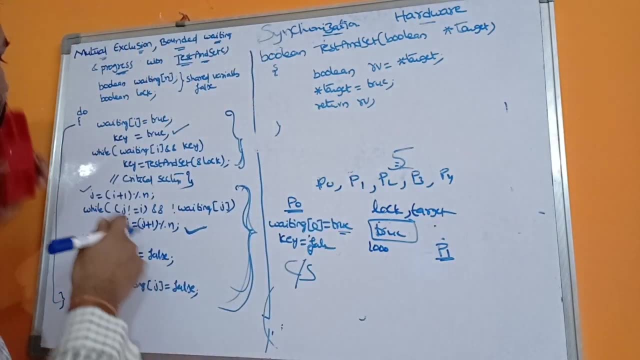 Then no other process is allowed to enter into the critical section. Let us assume that p1 process is interested to enters into the critical section, So p1 process entry section code will gets executed. Weighting of 1 is equal to 2.. 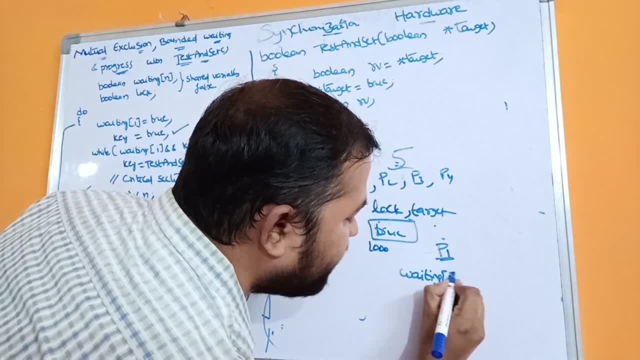 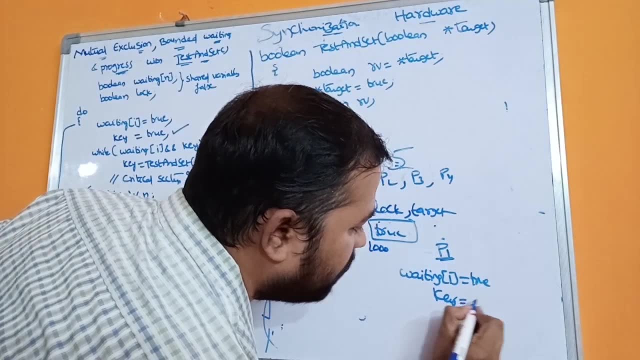 Weighting of i is equal to 2.. Here i value is 1.. So weighting of 1 is equal to 2.. And each process will have its own key variable. So key is equal to 2.. Next, this while condition will gets executed. 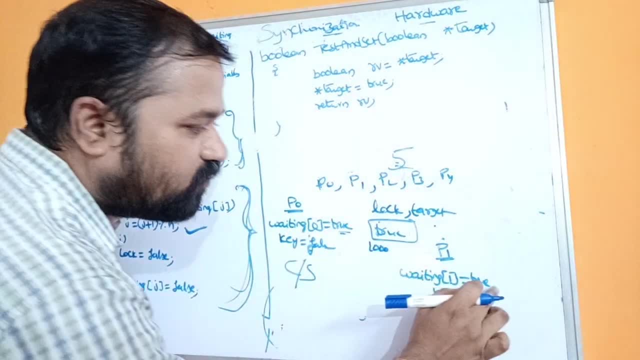 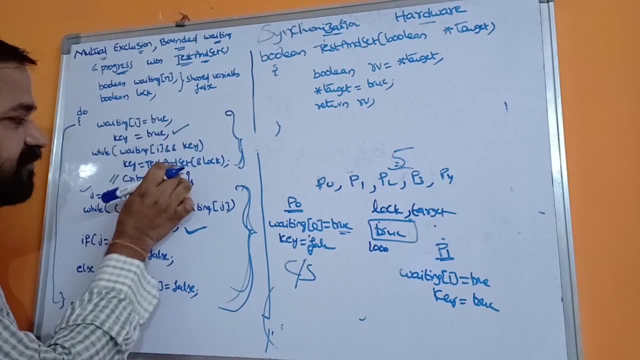 While weighting of 1.. So what is weighting of 1? True And what is key True. So both the conditions are true, So this body will gets executed. Key is equal to test and set of ampersand log. 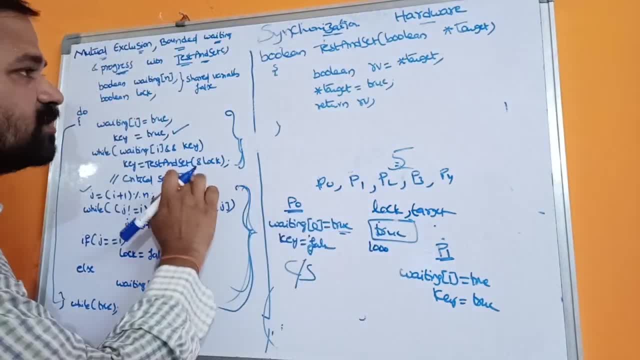 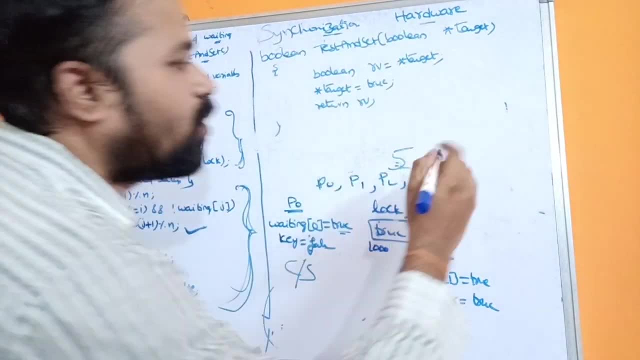 Log means 1000.. Ampersand log means 1000.. So this 1000 will be passed to target. Now target and log are pointing to the memory location 1000.. Boolean rb is equal to star. target rb is equal to what is the target here. 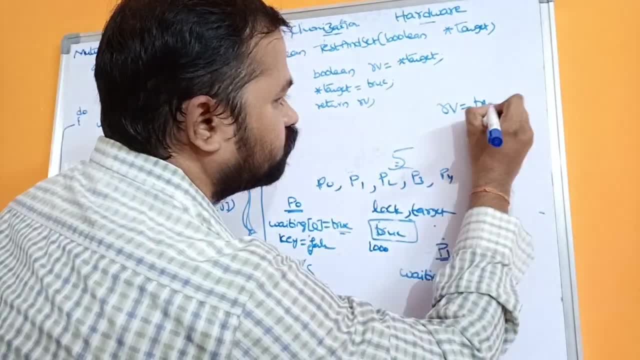 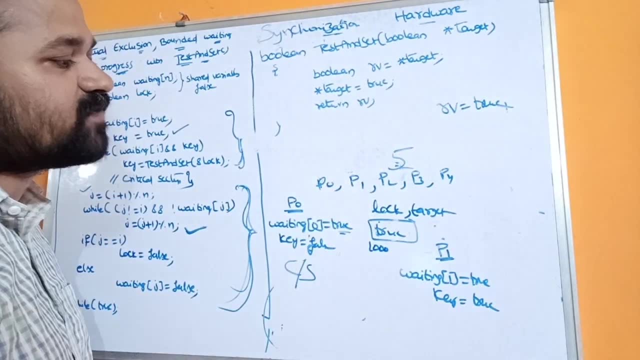 The value at the target Target is 1000.. rb is equal to 1000.. What is rb True? So rb is equal to true. Next star target is equal to true. Already target value is true only Return rb. 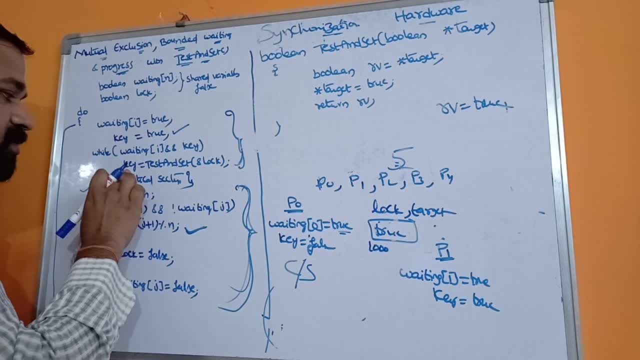 So this true will be written And it will be stored here. So now the value of the key is true. So once again, control goes to the while loop. So while weighting of 1.. Weighting of 1 is true. 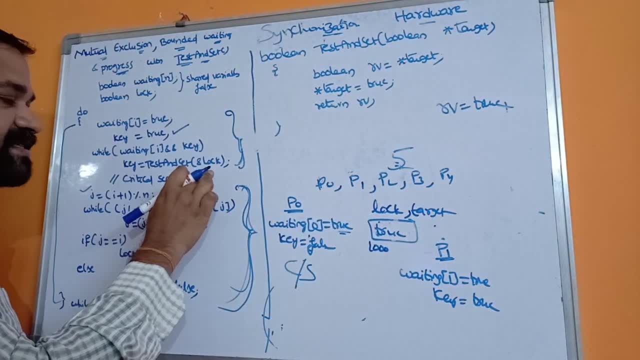 And key is true. So, once again, this body will gets executed. So likewise every time, while loop condition will become same. So likewise every time, while loop condition will become same. So likewise every time while loop condition will become same. 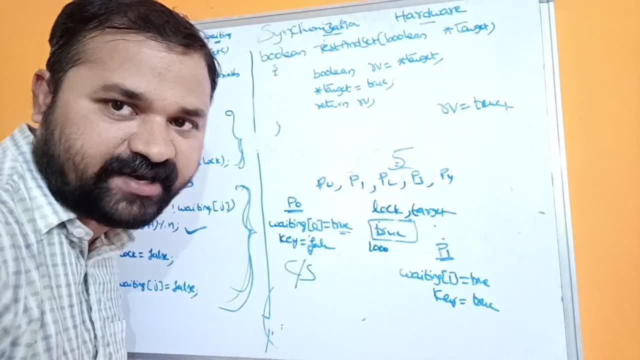 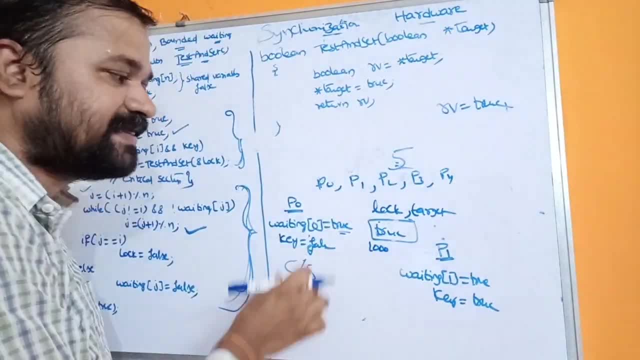 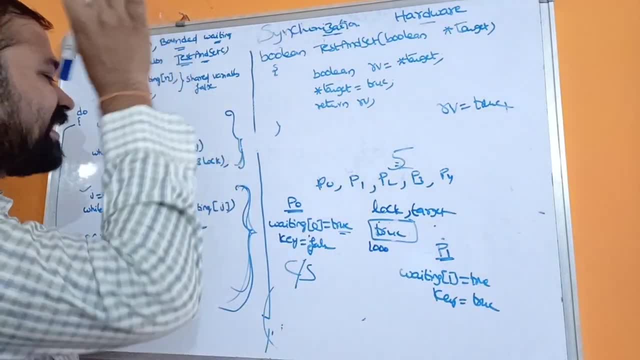 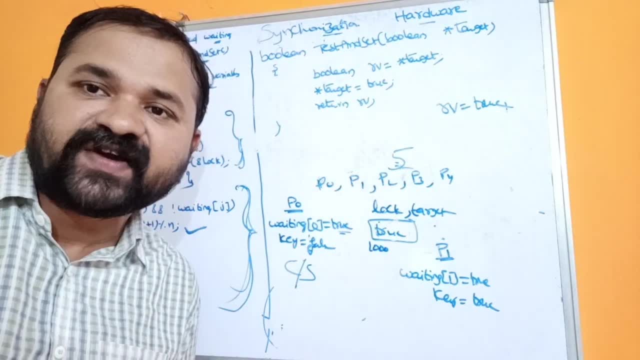 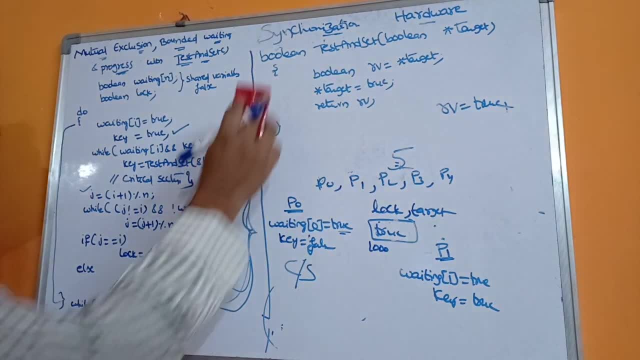 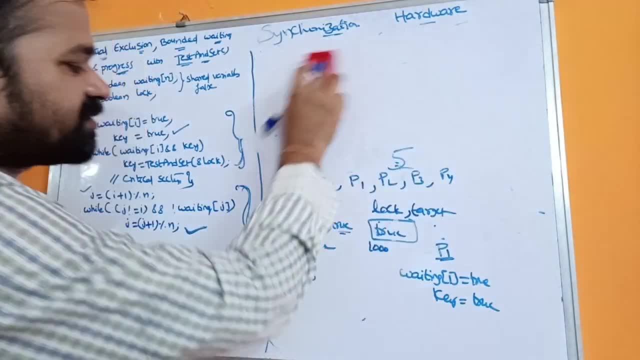 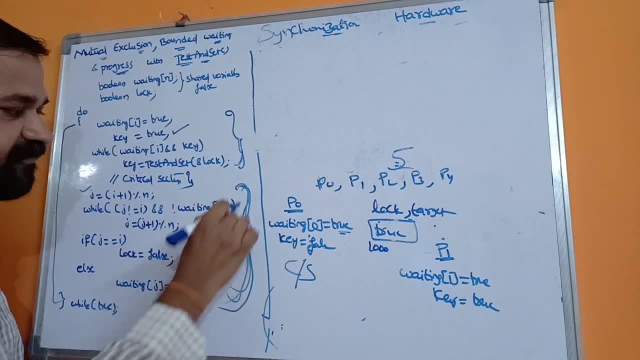 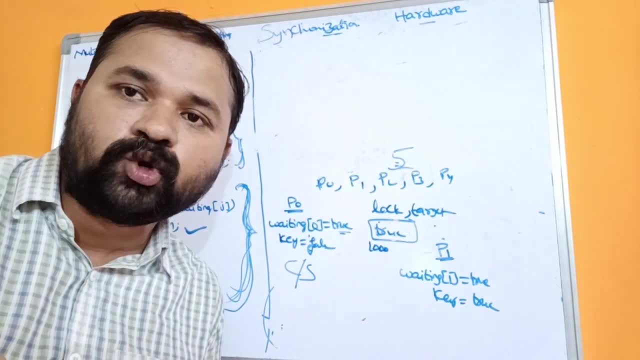 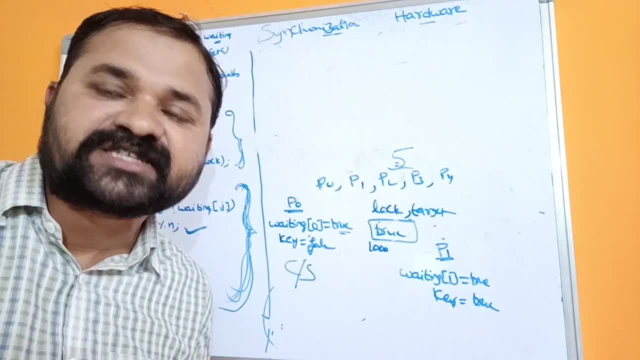 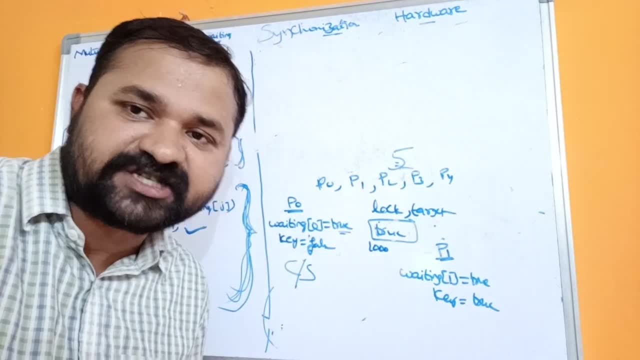 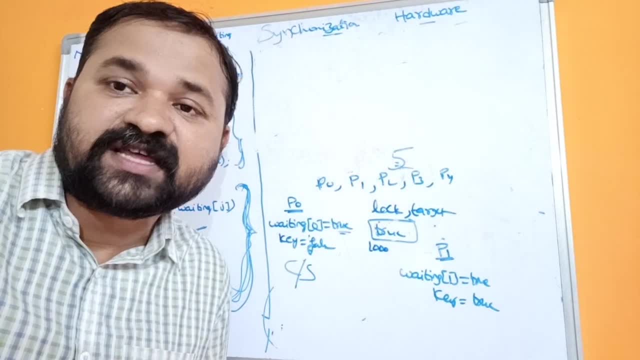 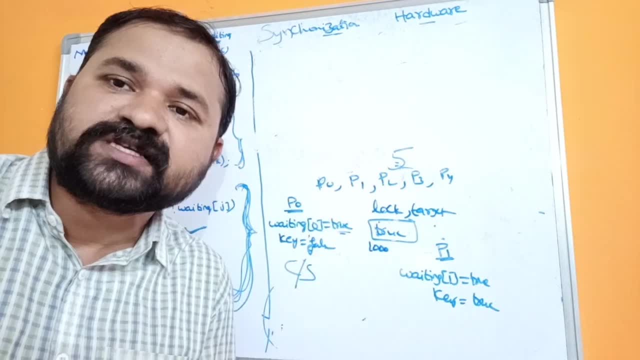 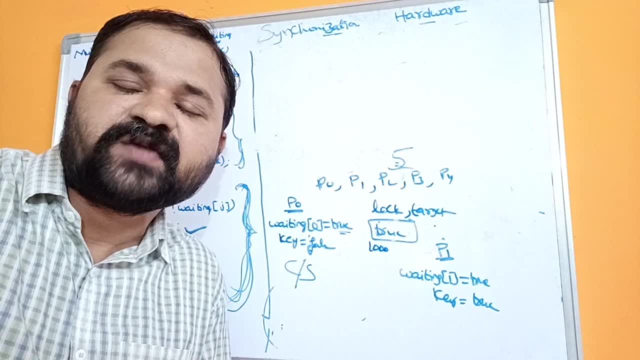 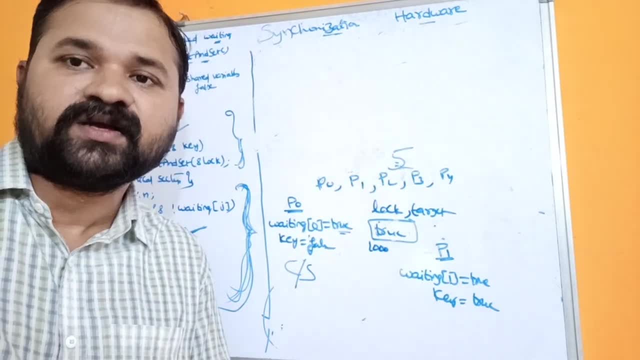 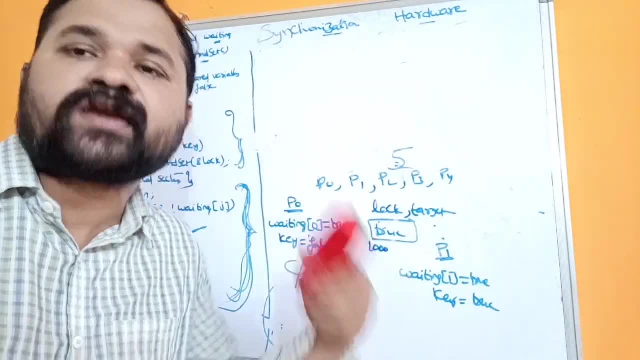 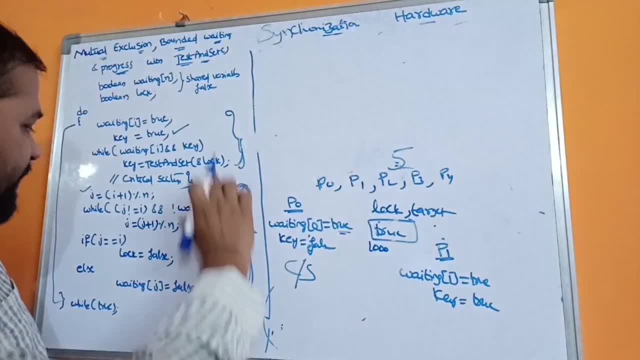 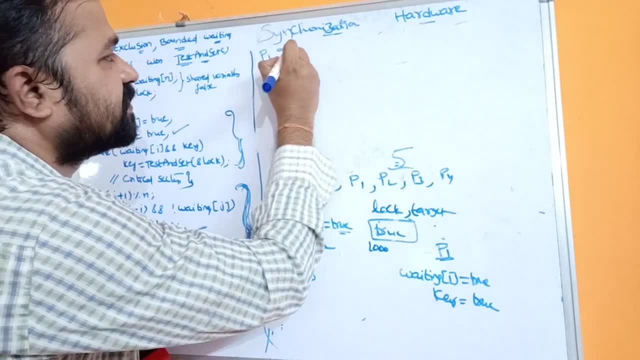 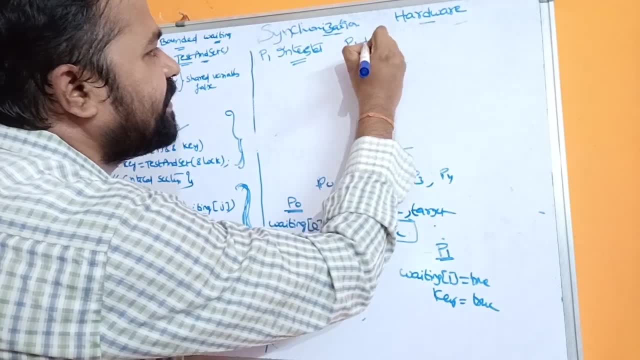 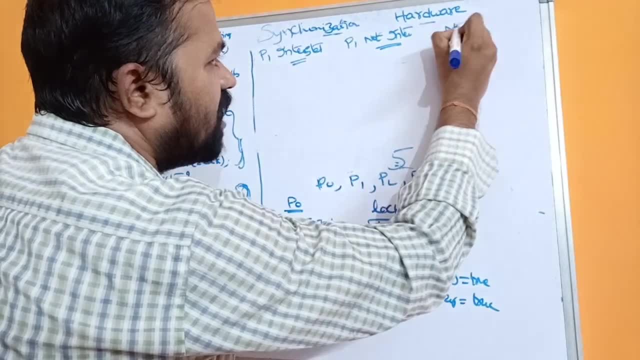 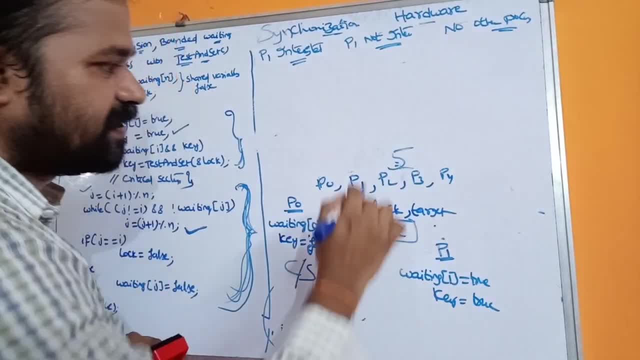 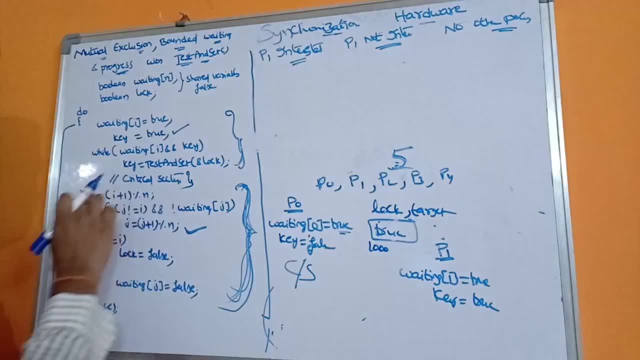 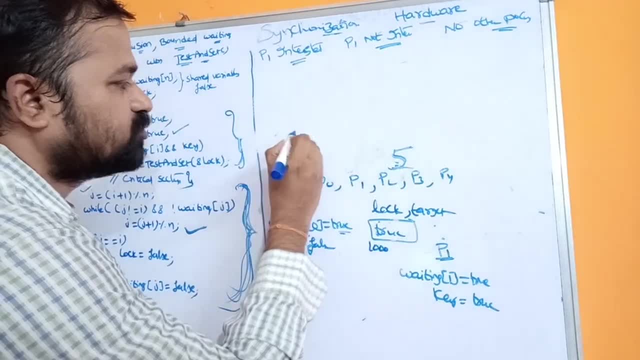 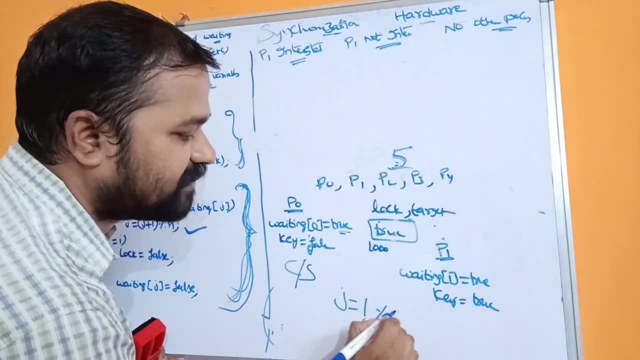 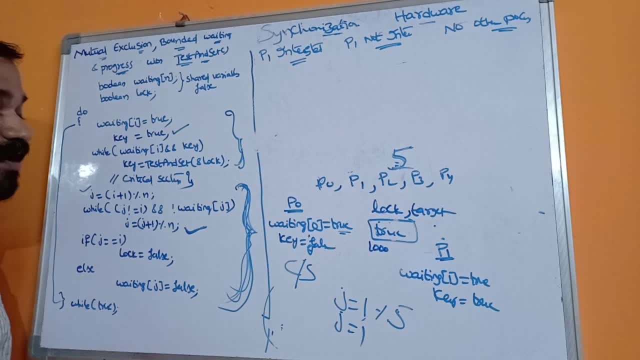 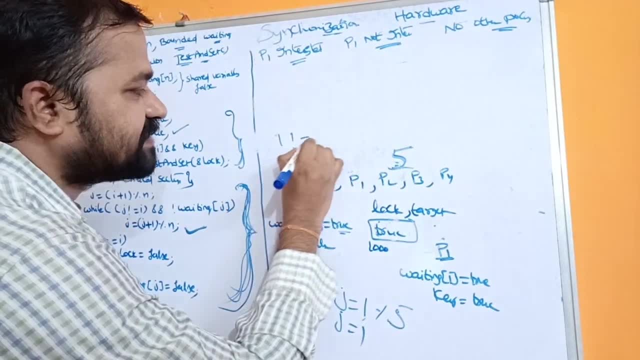 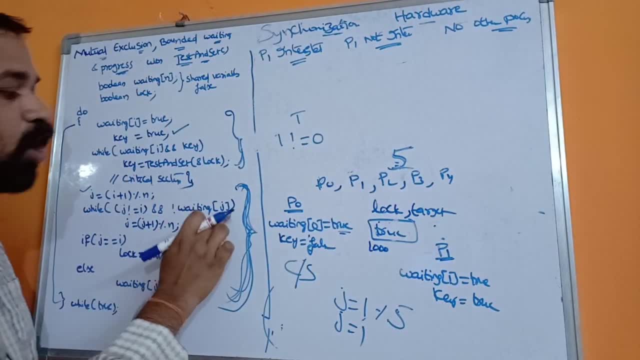 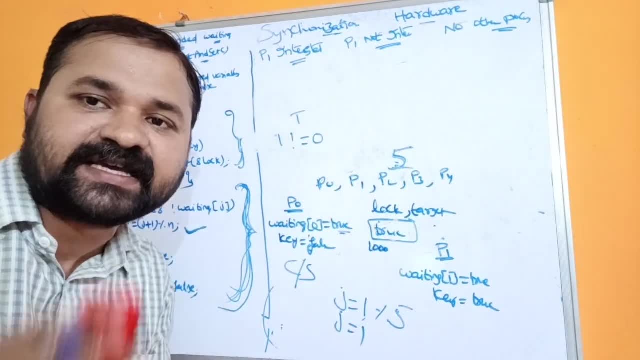 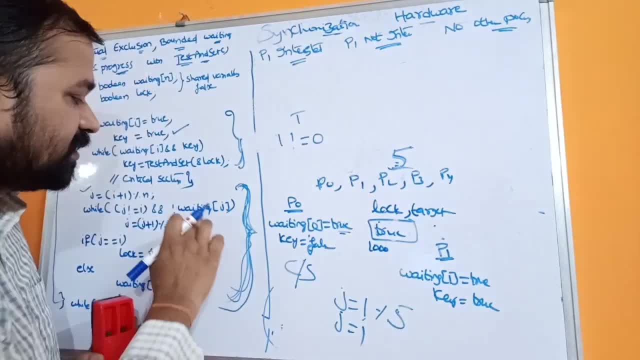 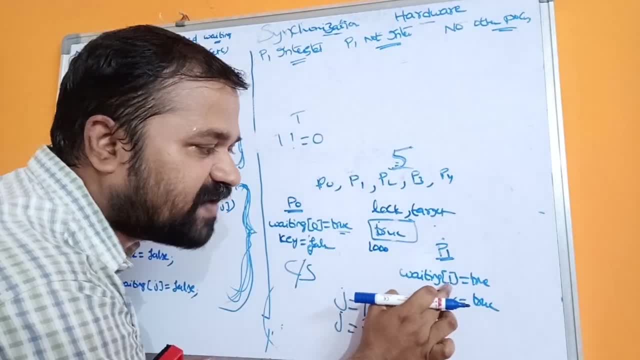 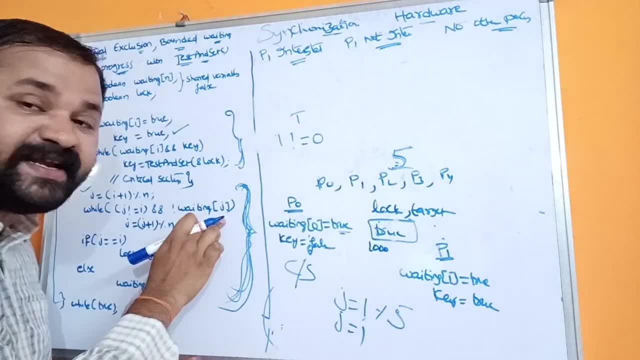 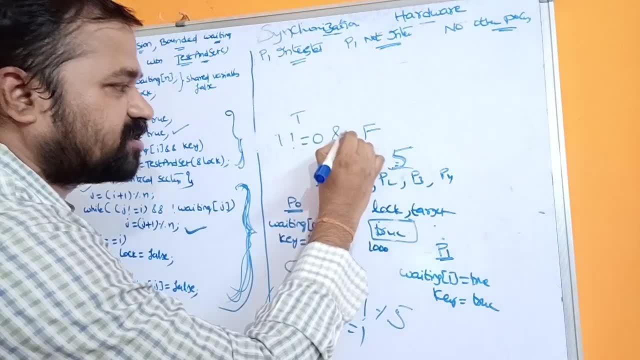 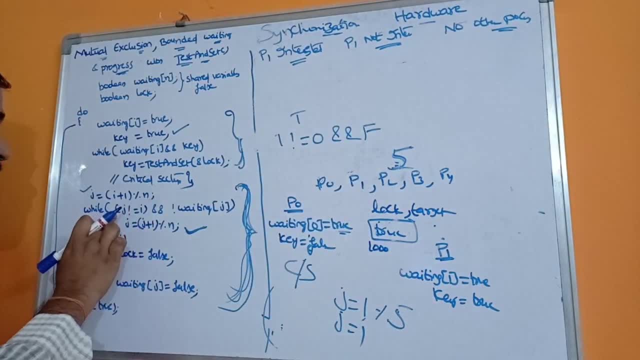 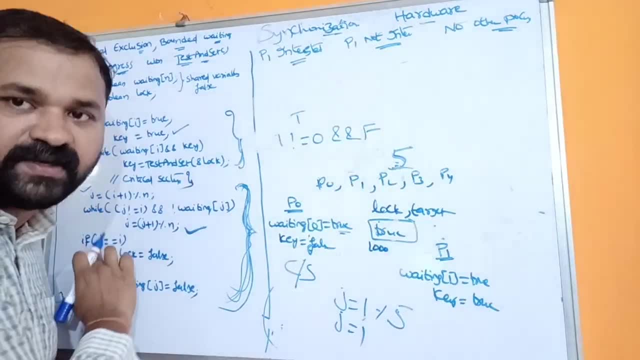 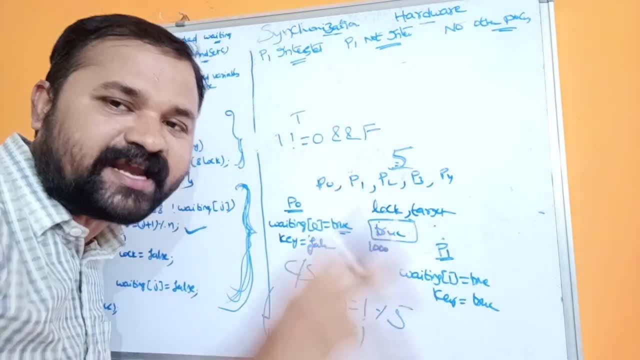 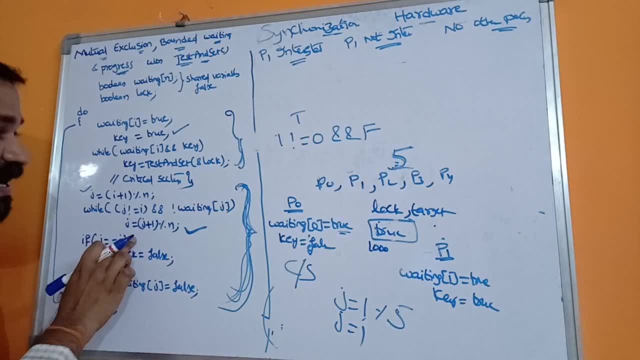 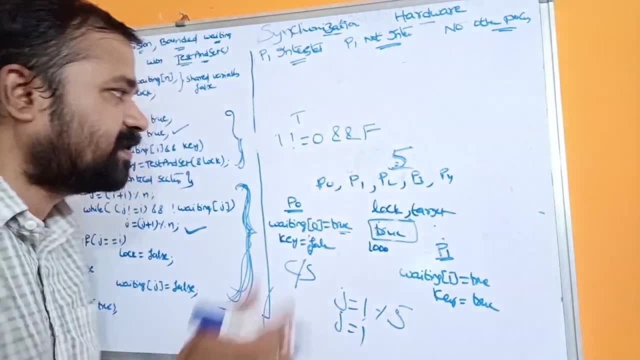 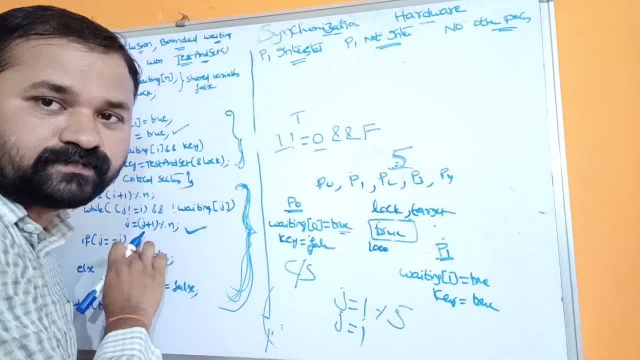 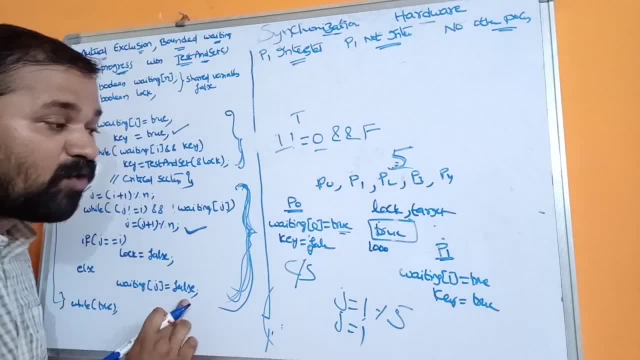 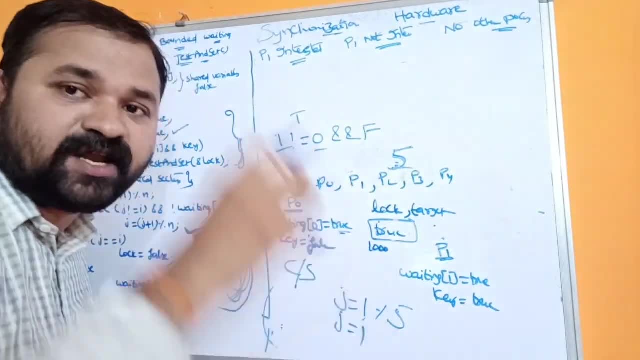 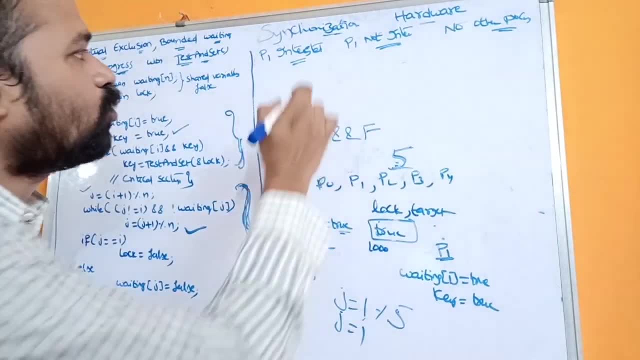 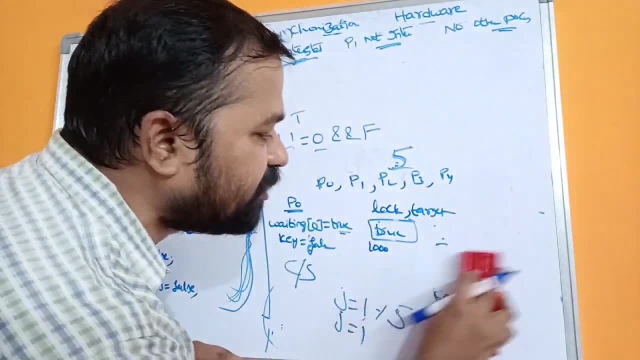 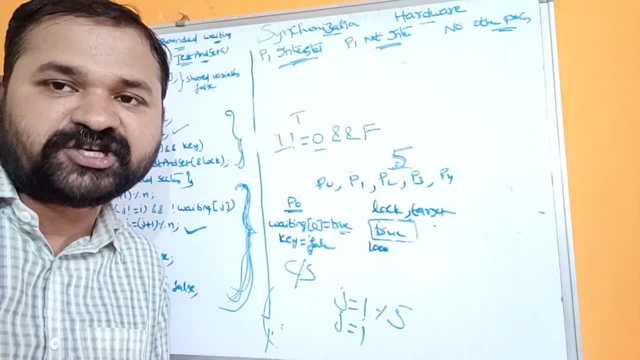 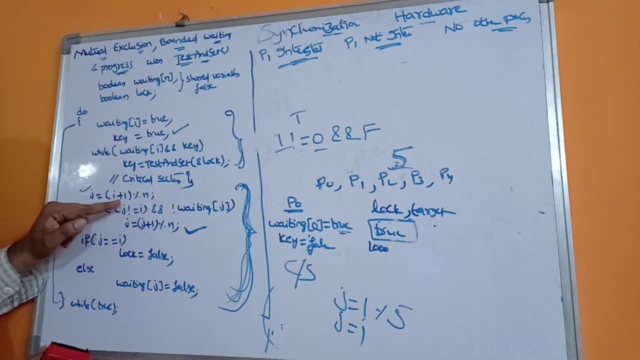 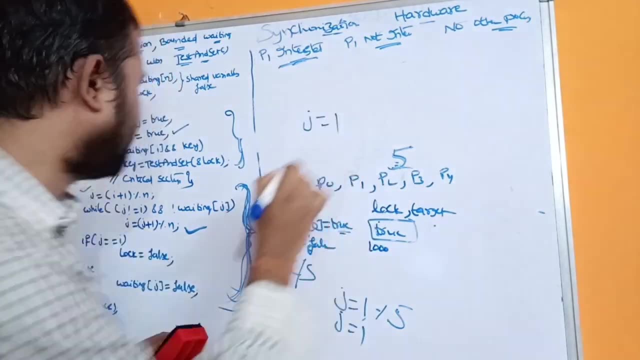 Okay, Further, let us check the code here. Okay, J is equal to I plus 1 modulo 1.. So what is J value? Already, we calculated J value is 1.. J value is 1.. Okay, 1 not is equal to 0.. 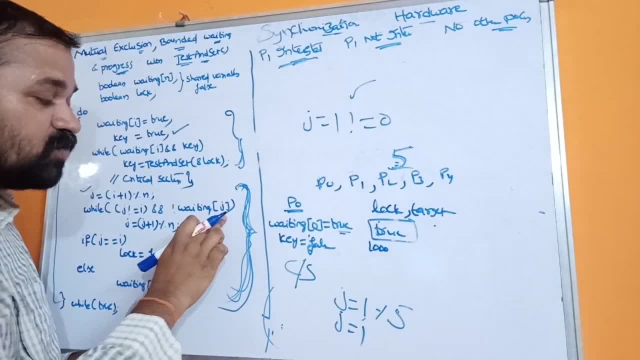 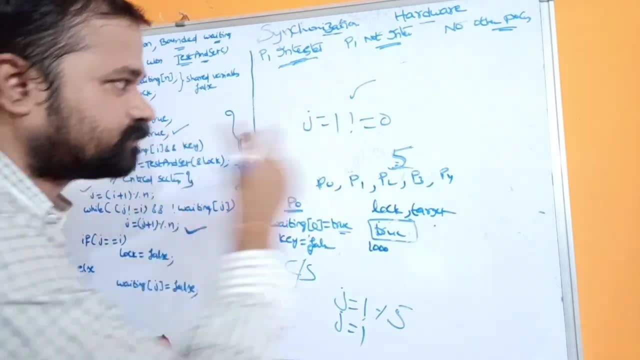 Yeah, Condition is 2.. Next, weighting of J. So what is weighting of J? Initially, all the values are false. Okay, So not false means what, 2.. Not false means 2.. So this is logical and both the conditions are true. 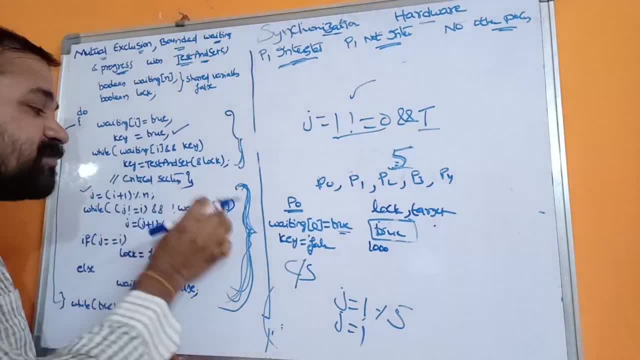 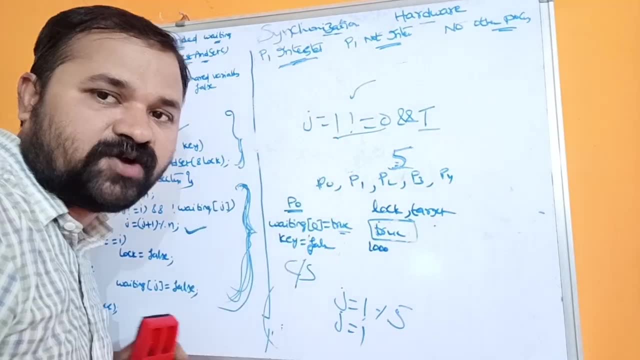 This condition is true, as well as this condition is true, So the entire expression will become true. So J is equal to J plus 1 modulo N. So what is the previous value in J? 1.. 1 plus 1 means 2.. 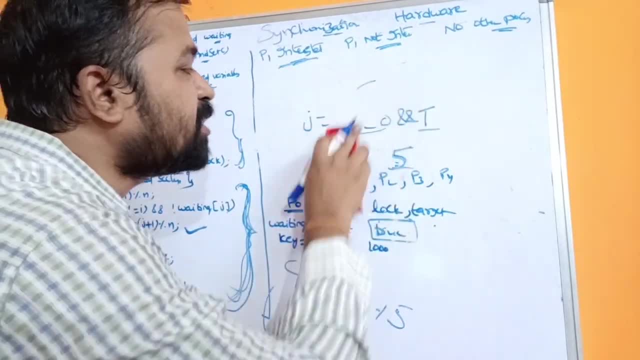 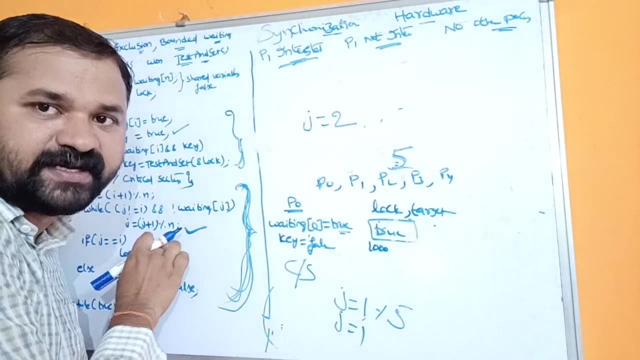 2 modulo 5 means 5. So that means P0 process is checking whether P2 is interested or not. So in that occasion this statement will get executed. If P1 is not interested, then it is checking whether. 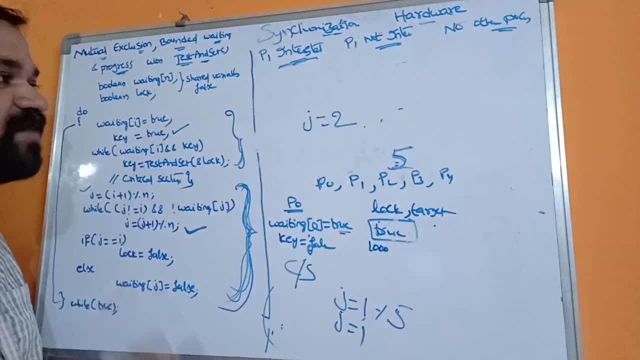 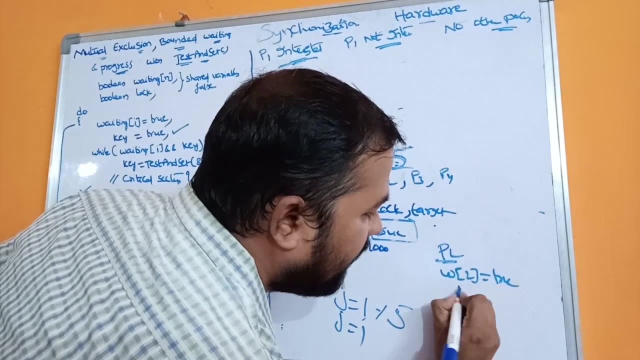 P2 is interested or not? Okay, So once again control goes to the value. So now, what is J? value 2. That means now P2 is interested. So weighting of 2 is true And its key value is true. 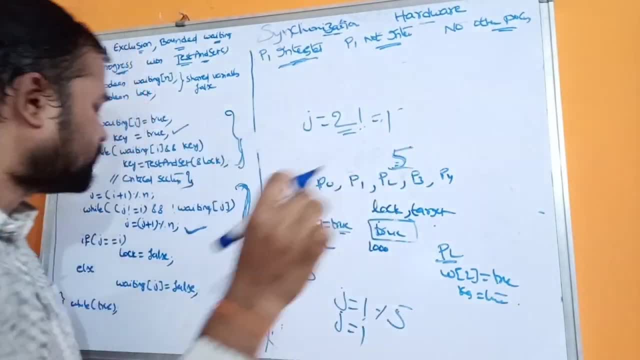 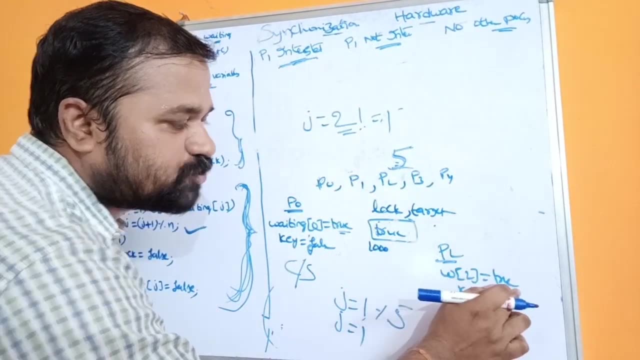 While J not equal to I, So 2 not equal to 1. Condition is true. Next, not weighting of 2.. What is weighting of 2?? Now, P2 is interested. So weighting of 2 means true. 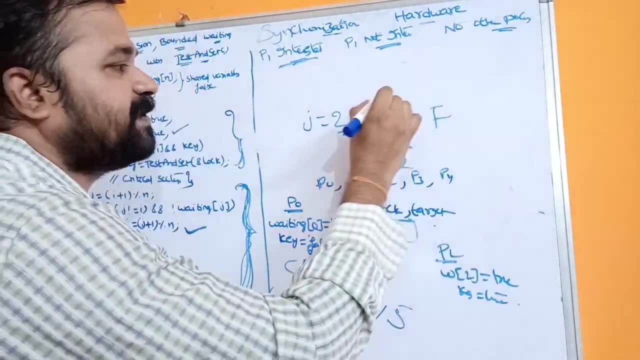 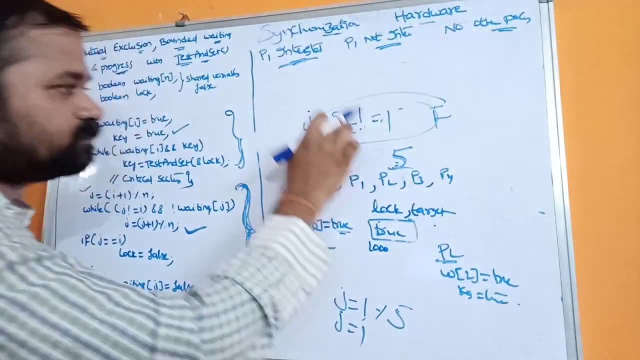 So not true means false, So true false. That means the entire expression is false. So the control comes out from the value. If J double is equal to I, J is 2, I is 0. Condition is false. 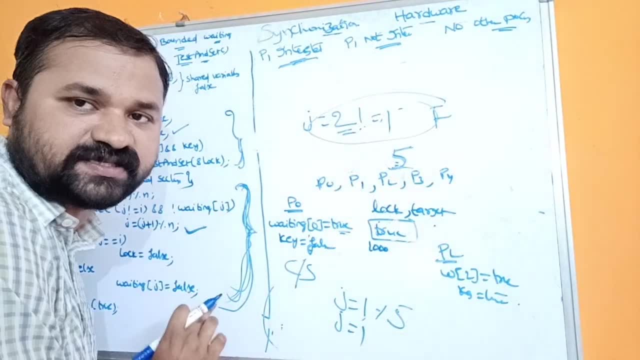 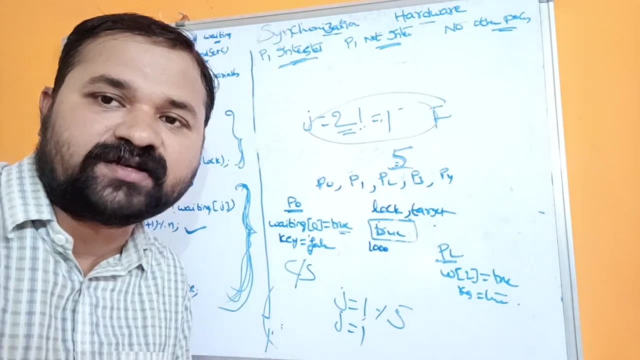 So else block will gets executed. Weighting of 2 is equal to false. So it means that now P2 process is interested into the critical section. So now P2 process will gets the chance to enter into the critical section. 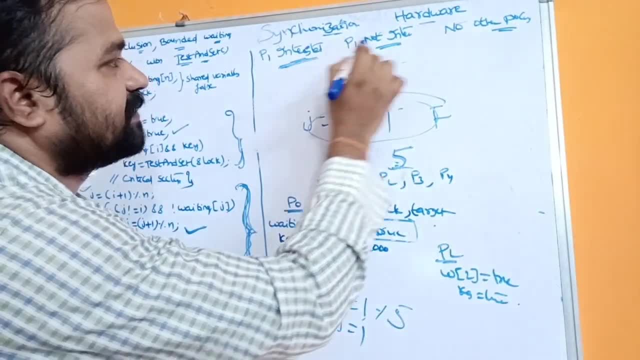 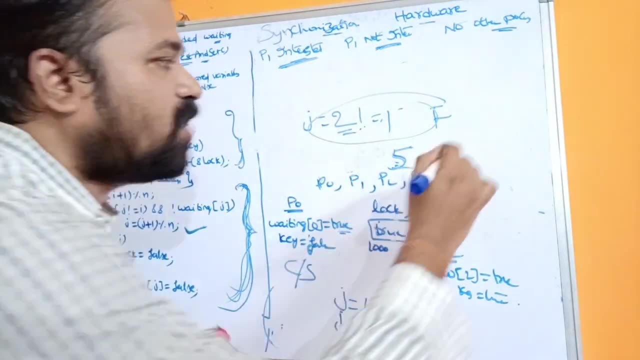 So with this we got complete idea about these two. Next, let us assume that no other process is interested in. to enter into the critical section, We have only one process, that is P0. So now N value will become what? 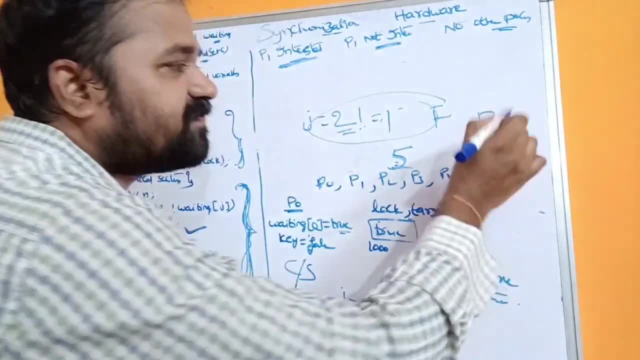 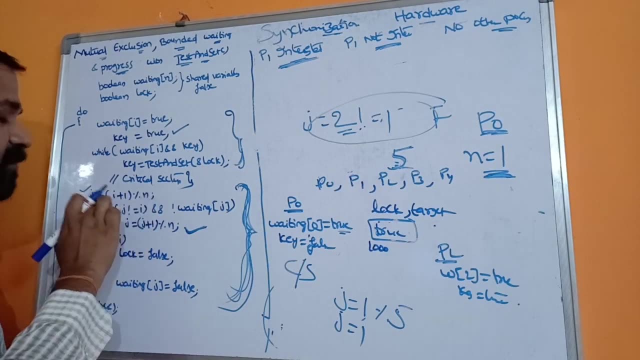 1.. If N value is 1, then it specifies that we have only one process, So that process only will enter into the critical section. J is equal to I plus 1 modulo N. What is I value 0.. 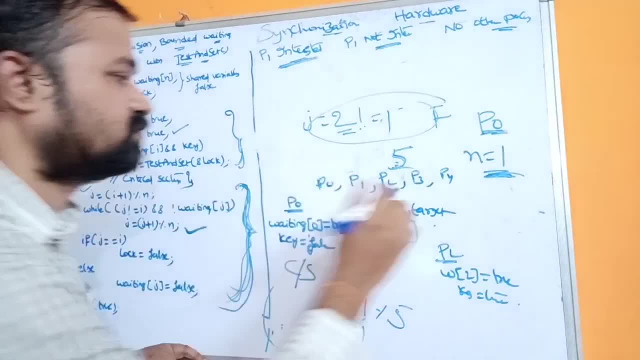 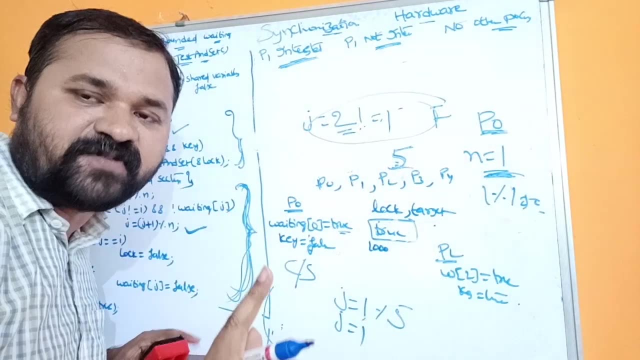 0 plus 1 means 1.. 1 modulo What is N value? now N value is 0.. So 1 modulo 1 means 0.. So now J value is 0.. Why? Because there is only one process. 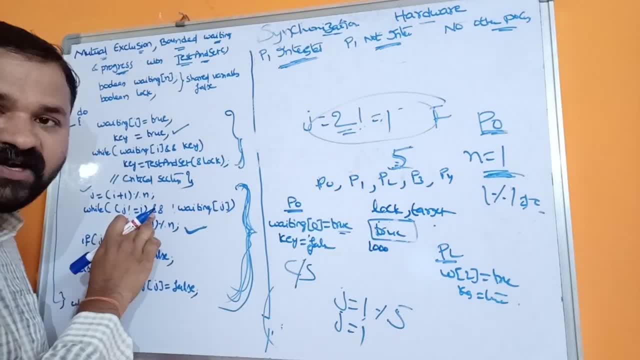 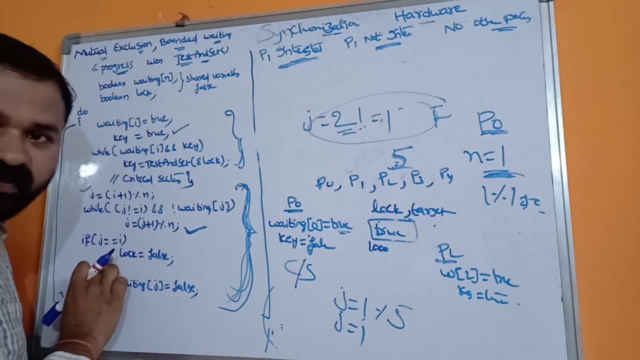 That is interested to enter into the critical section. While J is not equal to I, J value 0, I value 0.. 0 is not equal to 0. Condition is false, So the control comes out from the while loop. 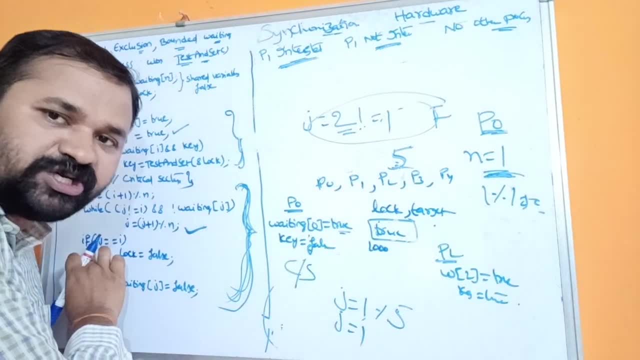 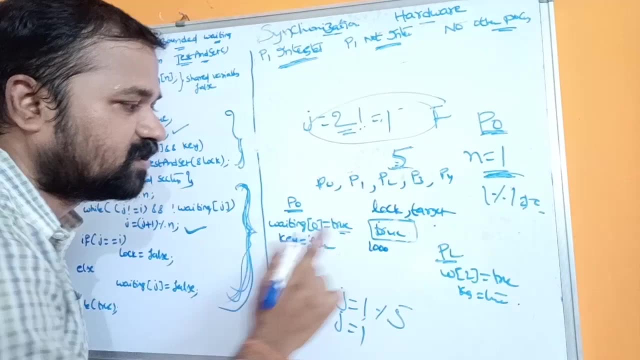 Okay. Next, if J double is equal to I, J value 0, I value 0. So both the conditions are true. J is 0, I is 0. True, So log is equal to false. So now log value will be set to false. 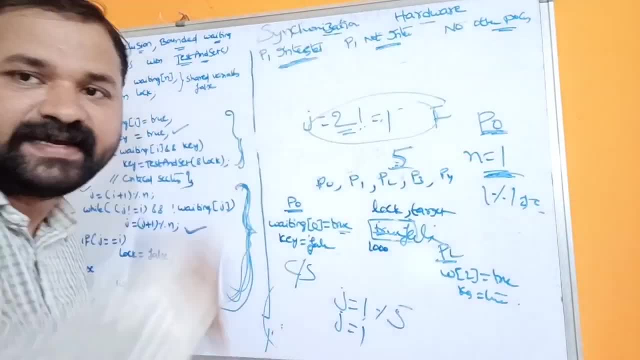 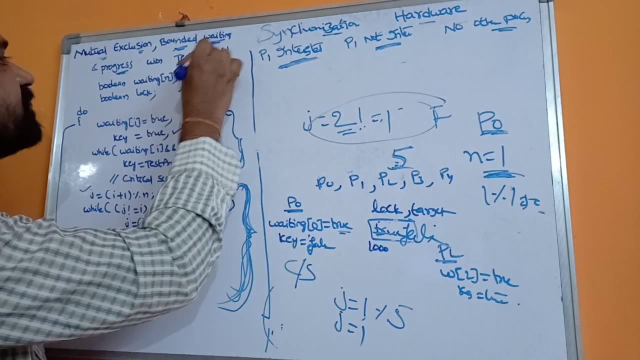 So that now, if P0 is interested, then P0 process can enter into the critical section. So this is the code for exit section. Now let us check whether this algorithm is satisfying bounded weighting and progress or not. We know what is bounded weighting. 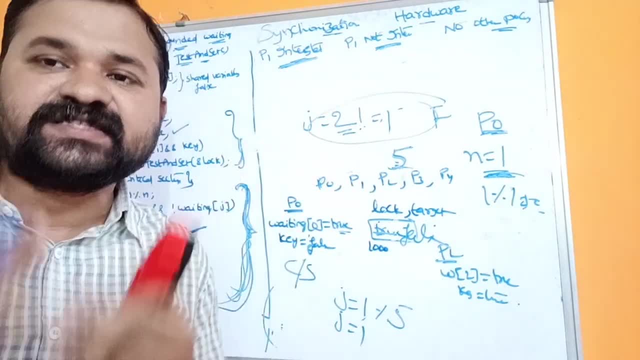 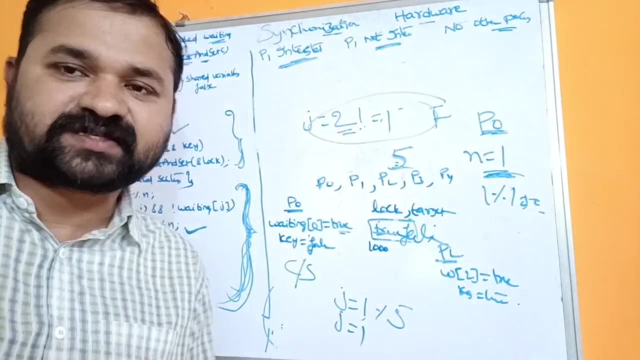 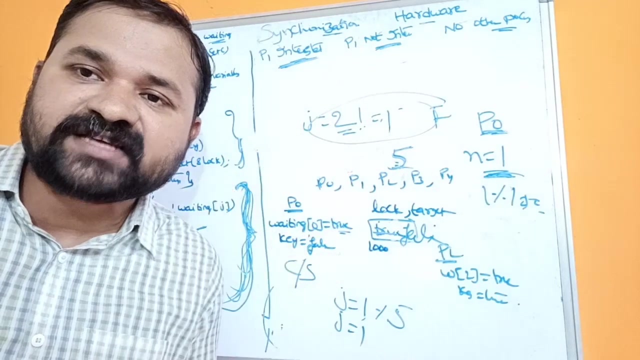 Each process has to get a sufficient number of chances to enter into the critical section. Only one process cannot enter into the critical section for many number of times. Here what P0 is doing: Whenever P0 process comes out from the critical section, it is checking whether P1 is interested or not. 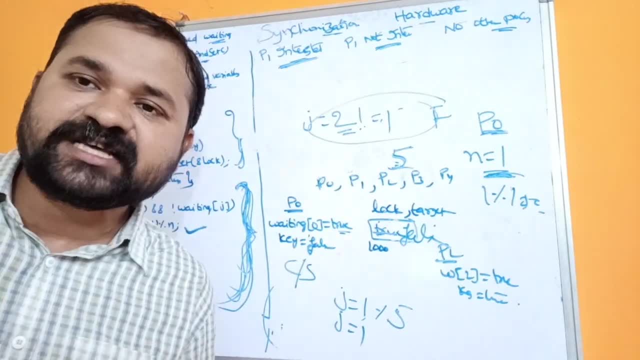 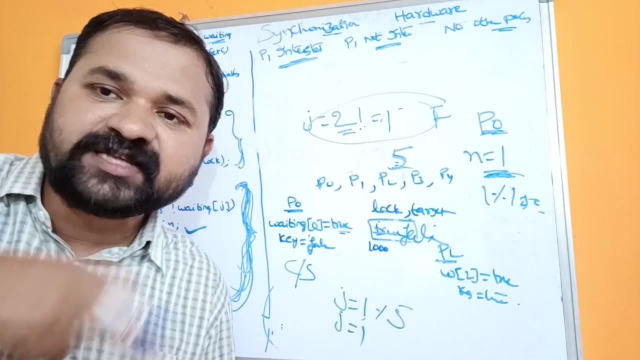 It is checking whether P2.. If P2 is interested or not, it is checking whether P3 is interested or not. So that means here each process can check the remaining all other processes. Let us assume that P1 process is in the critical section. 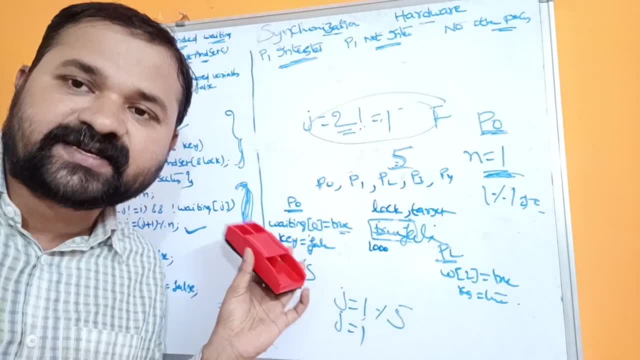 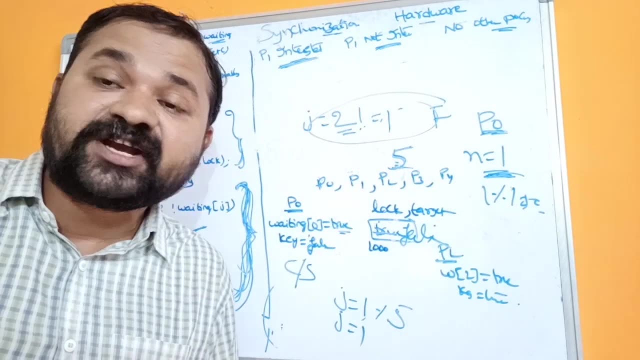 So while P1 process is coming out from the critical section, P1 process will check whether P2 is interested or not. If P2 is not interested, then it will check whether P3 is interested or not. So here each process will get sufficient number of chances. 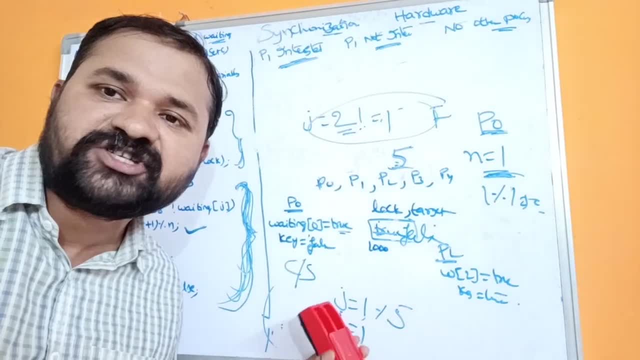 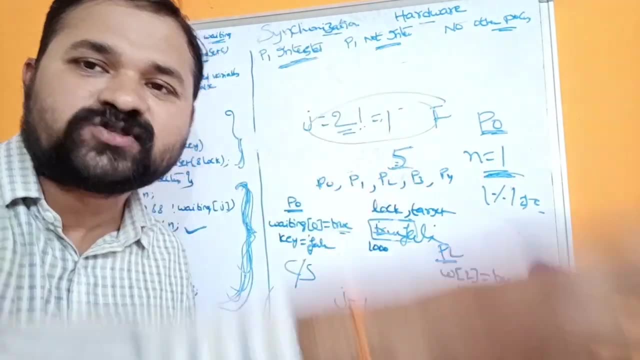 At a time, only one process cannot enter into the critical section, So we can say that this algorithm will satisfy bounded weighting. There is a limit on number of times a process can enter into the critical section. If P1 is interested, then no problem. 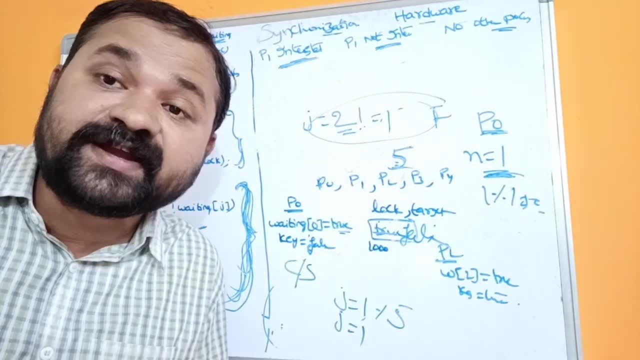 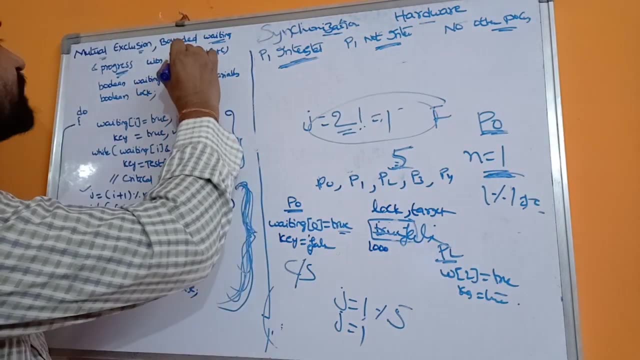 P1 process comes into the critical section. If P1 is not interested, if no other process is not interested, then only P0 process can come into the critical section. So we can say that it is satisfying bounded weighting. And last one is progress. 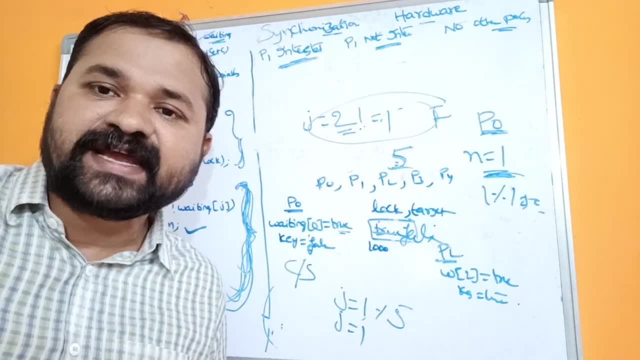 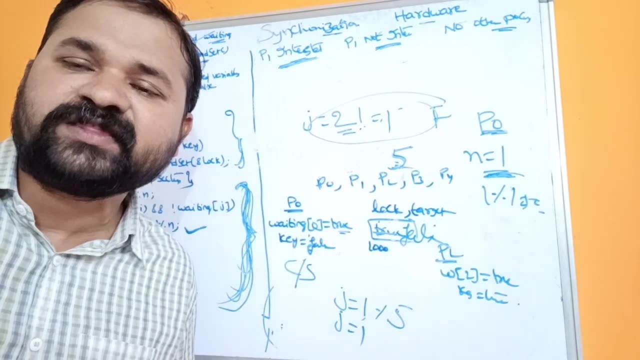 Progress means the decision about which process can enter. So the decision about which process can enter into the critical section will be taken in a finite amount of time. Here P0 is checking for P1,, P2,, P3, P4..